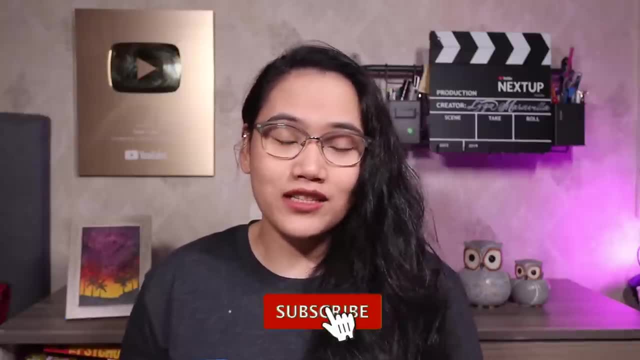 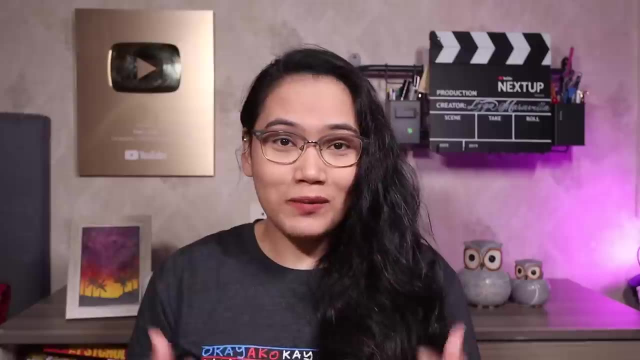 content. So if you don't want to miss any of my uploads, don't forget to hit subscribe and hit that bell icon. Now, like I said in the intro earlier, we're going to talk about arithmetic sequences. The main topic is the formula, how to solve it, etc. But before we do that, just a quick. 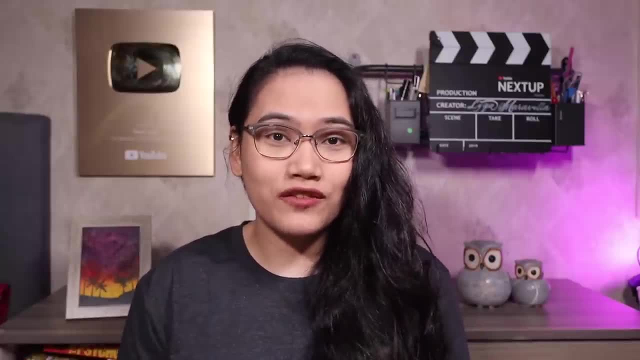 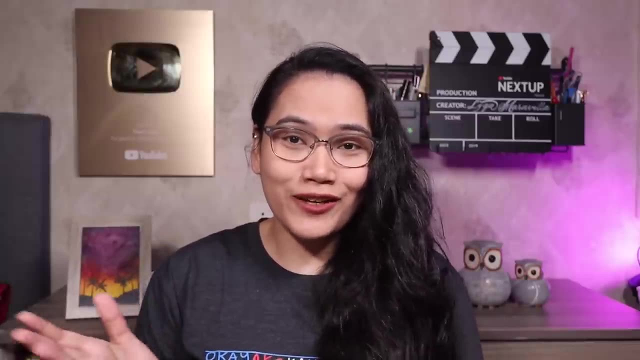 little plug. if you want to help support our channel and our cause to democratize education in the Philippines, One way that you can do that is by being a channel member. So all of our channel members today. thank you so much to all of you. I hope you don't mind me giving you a quick shout. 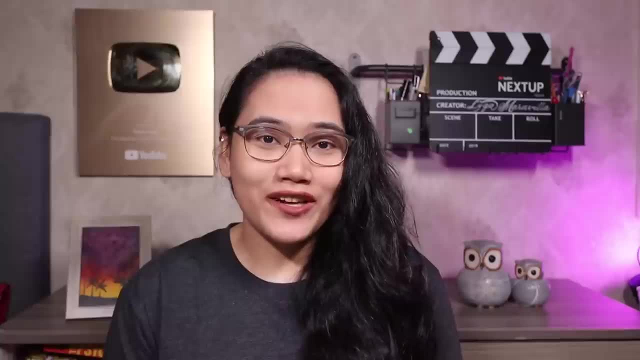 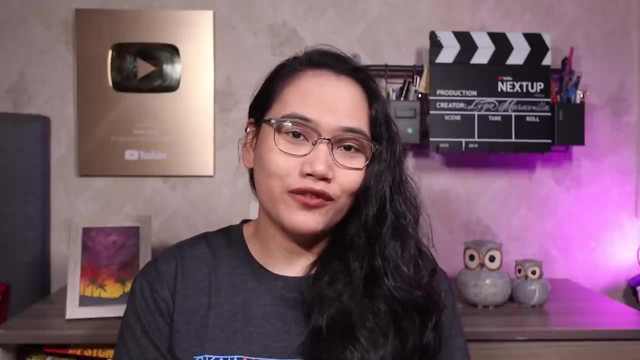 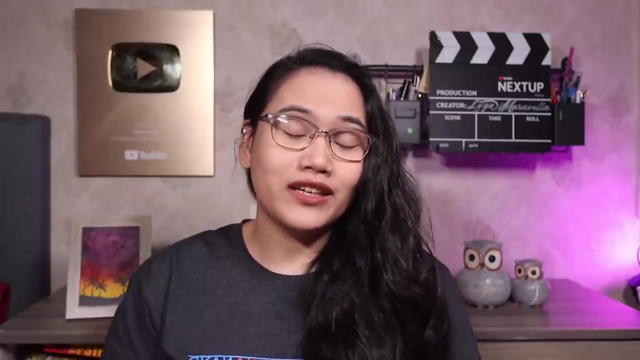 out today. Thank you for helping keep the lights on this operation and making sure that we have enough to pay the bills, etc. and even grow the team. So thank you for your contribution. Thank you for helping me help more people through this channel. If you want to volunteer and send your support, 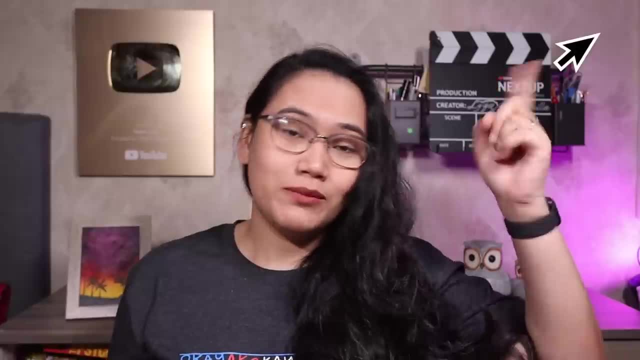 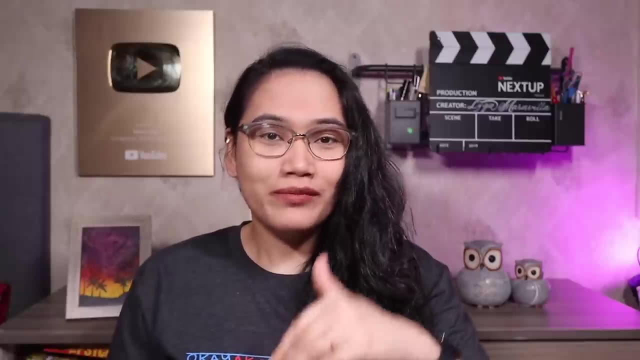 as a channel member. you can click on the i button here for the explainer video, or you can click on the join button beside the subscribe button if you're watching on YouTube to find out which tier works for you. All right, so thank you again. 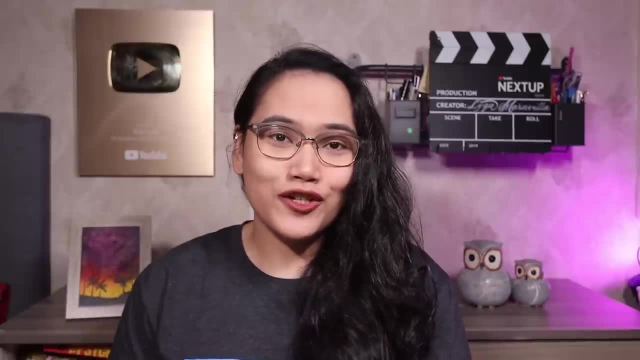 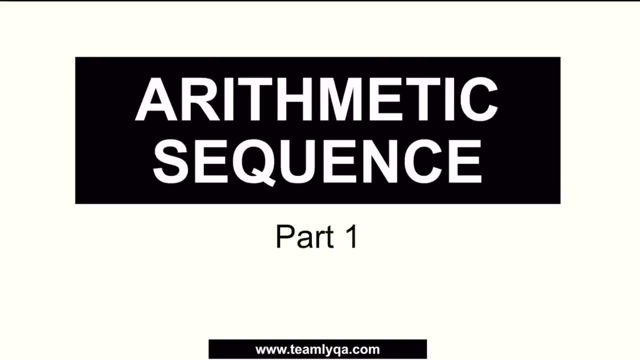 As we turn our tablet for this discussion. I just want to appreciate all of you all, right? Yeah, I'll see you in a bit, And in this video we're going to talk about the炎ArTHEs firs and how can use the formula. 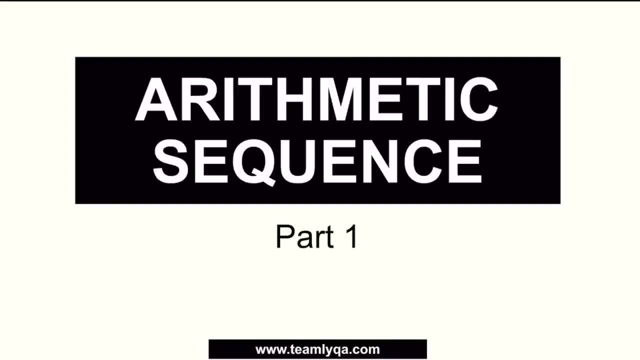 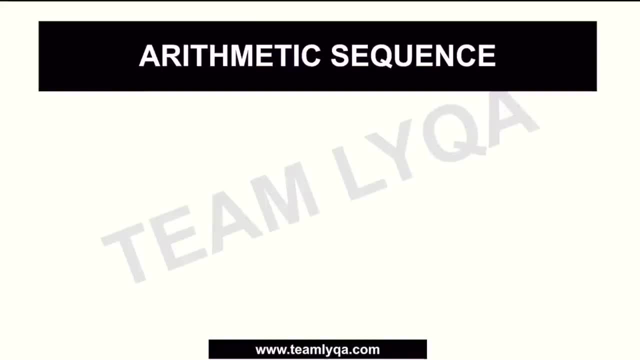 and when there comes a term 말이able or not and other termsários. Now the first thing we need to do is to define what an arithmetic sequence is, And the real definition of a formula might be something similar. here You can use it different ways. 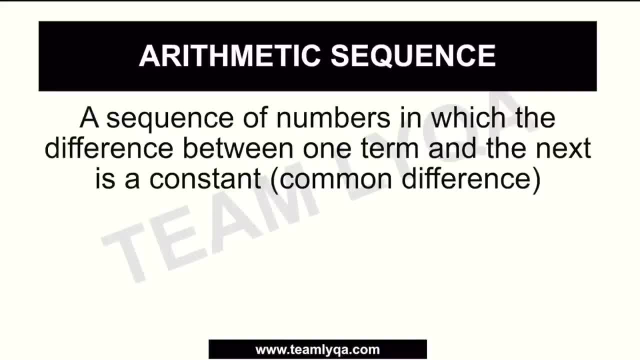 like, for example, in Catalog, and multiplicity and so on, But no need to stand around here for this if you still have questions on that. So let us summarize because I'm not sure if you understood, And to keep it simple: it's a sequence of numbers in which the difference between one term and the next is a constant. 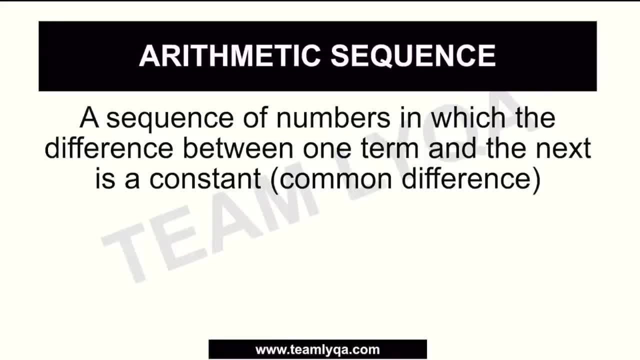 So we also call this a common difference. Again, it's a sequence of numbers like these. Then the difference, or the difference between one term and the one that follows it should be a constant. Okay, now, how do we check that? 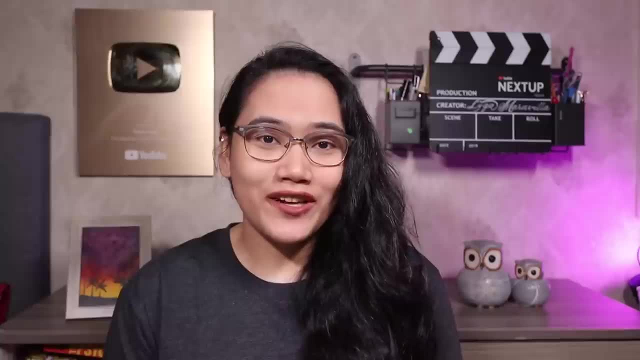 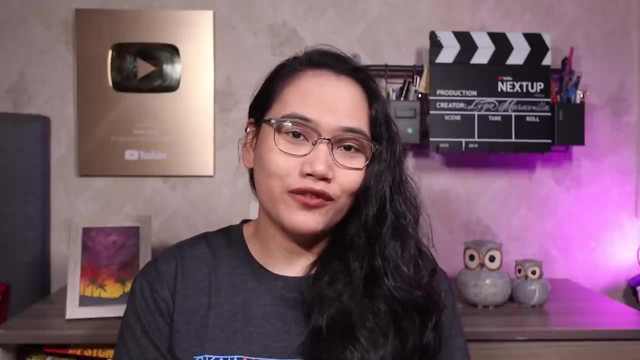 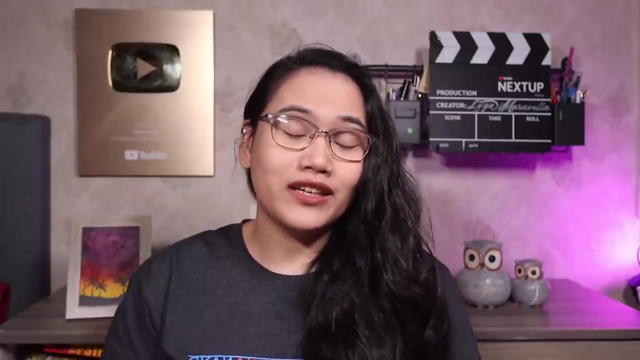 out today. Thank you for helping keep the lights on this operation and making sure that we have enough to pay the bills, etc. and even grow the team. So thank you for your contribution. Thank you for helping me help more people through this channel. If you want to volunteer and send your support, 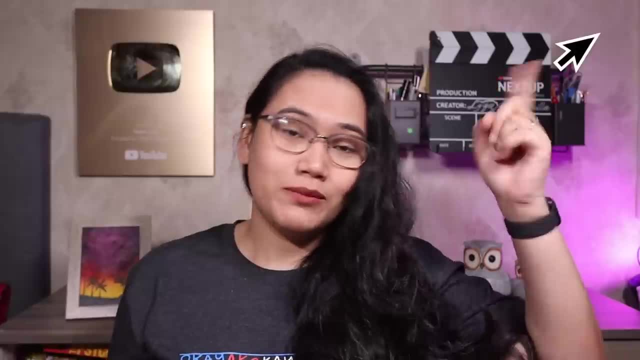 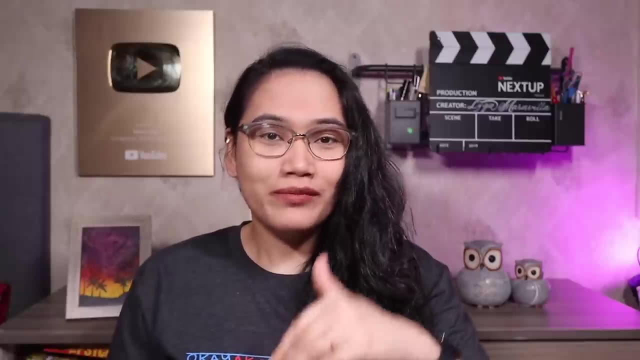 as a channel member. you can click on the i button here for the explainer video, or you can click on the join button beside the subscribe button if you're watching on YouTube to find out which tier works for you. All right, so thank you again. 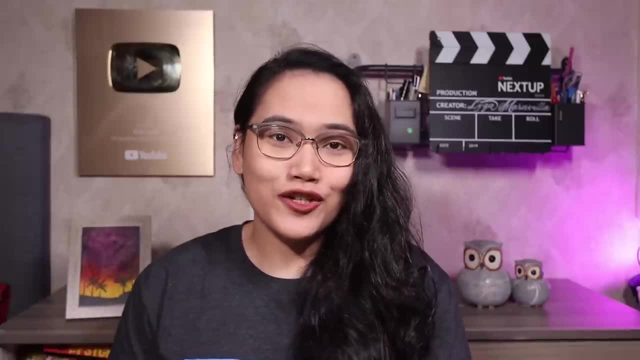 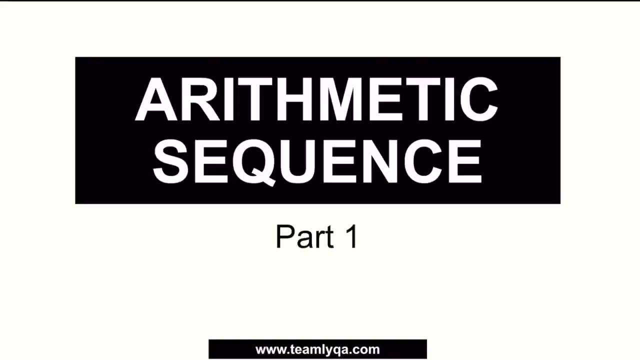 Thank you for supporting us. I hope you enjoyed this video And, as we turn to our tablet for this discussion, I just want to appreciate all of you. All right? Yeah, I'll see you in a bit, All right? So this is our lesson on arithmetic sequence, And in this video we'll talk about 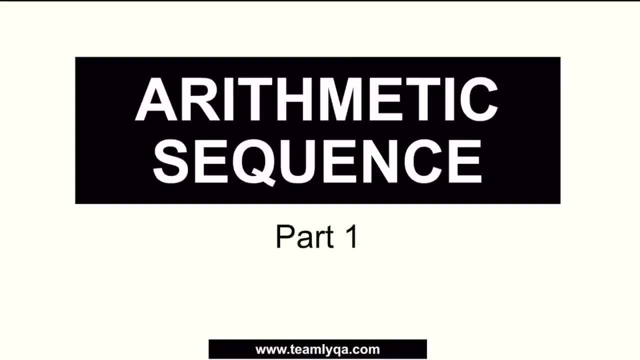 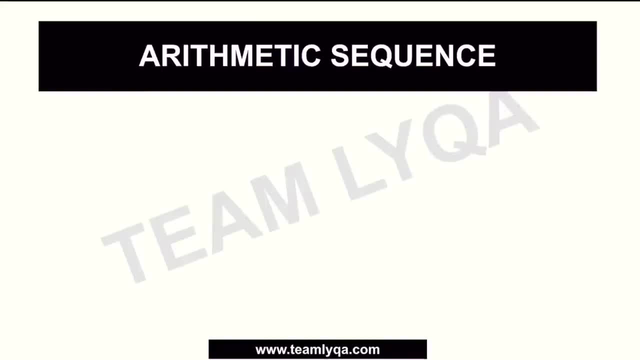 what it is, how to get the formula and how to use the formula. if there are any terms that are missing, or if the initial term is missing and many others, okay, Now the first thing you need to do is to define what an arithmetic sequence is, And I hope you enjoyed the video. If you enjoyed it, please don't forget to like and subscribe. Thank you so much. Bye-bye. 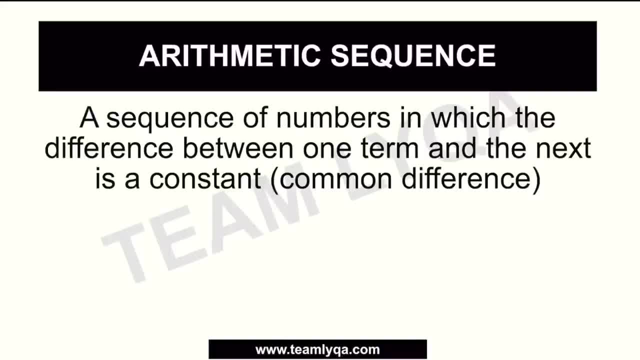 to keep it simple, it's a sequence of numbers in which the difference between one term and the next is a constant, So we also call this a common difference. Again, it's a sequence of numbers like these: Then the difference, or the difference between one term and the one that follows it. 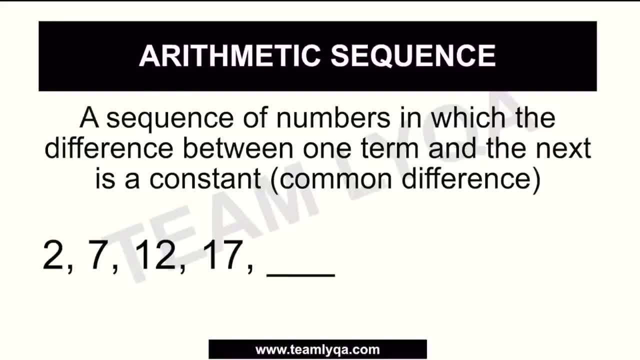 should be a constant. Okay, now, how do we check that? One thing that we can do is just look at the gaps. So ang 2 to 7,, that is plus 5.. Ang 7 to 12, magpa-plus ka rin ng 5.. Now ang 12 to 17,. 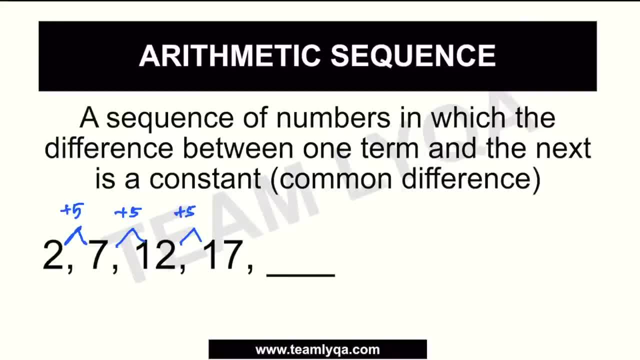 plus 5 din. So it's safe to assume na ang susunod na number dito is yung dadagdagan din natin ng 5.. Now himayin natin ng kaunti itong mga terms na ginagamit natin. The first one is yung: 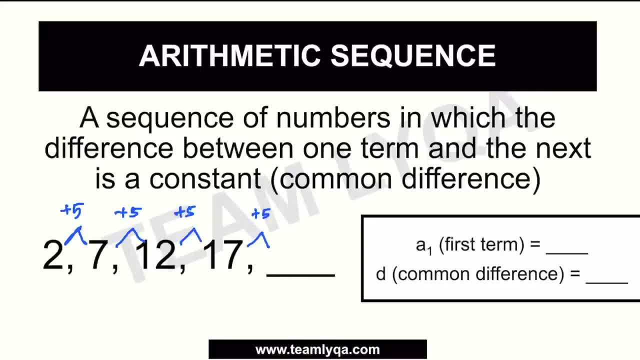 tinatawag nating first term. Ano ba yung term? Ang term ay itong mga numbers na ito. Now ang first term is this: Okay, yung nauuna dun sa listahan. Now, in this case, ang first term is 2.. So ilalagay lang natin. 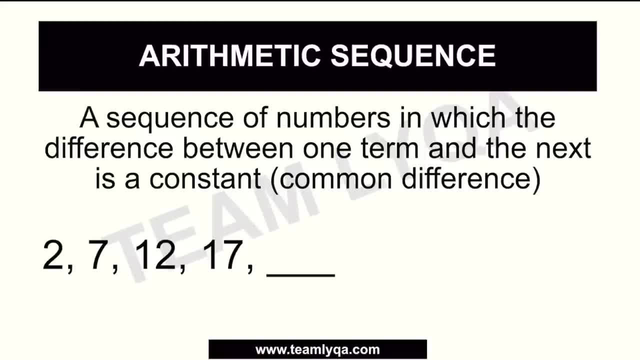 One thing that we can do is just look at the gaps. So ang 2 to 7,, that is plus 5.. Ang 7 to 12, magpa-plus ka rin ng 5.. Now ang 12 to 17, plus 5 din. 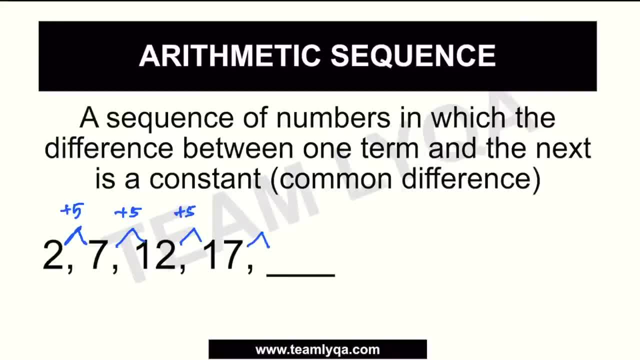 So it's safe to assume na ang susunod na number dito is yung dadagdagan din natin ng 5.. Now himayin natin ng kaunti itong mga terms na ginagamit natin. 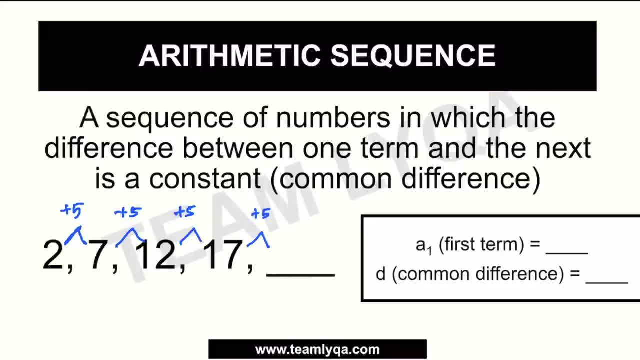 The first one is yung tinatawag nating 5.. First term: Ano ba yung term? Ang term ay itong mga numbers na ito. Now, ang first term is this: Okay, Yung nauuna dun sa listahan. 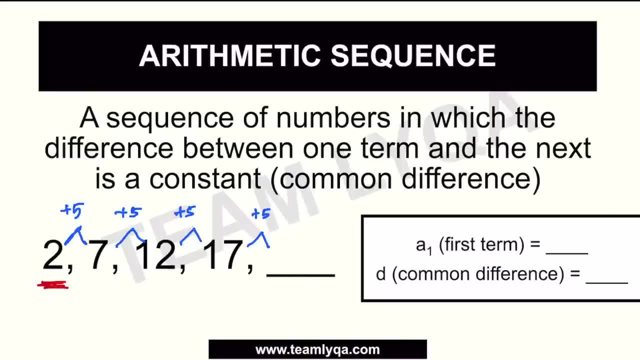 Now, in this case ang first term is 2.. So ilalagay lang natin siya dito. Now, why is it important? Kasi mamaya sa formula dapat automatic sa atin yung pag-spot ng mga yan. 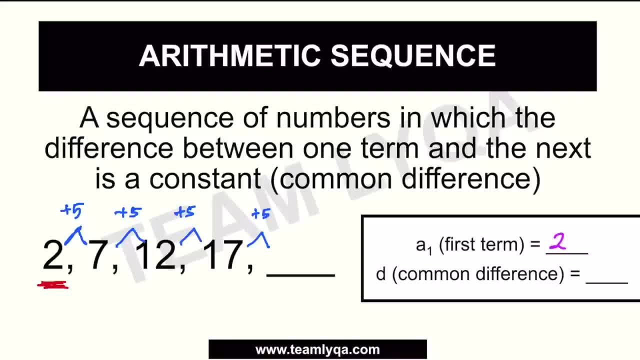 Now yung d naman is what we call the common difference, Yun yung constant na pinagkaiba ng mga numbers na yan. Sa case na ito, that is plus 5.. Again, pare-pareho sila. 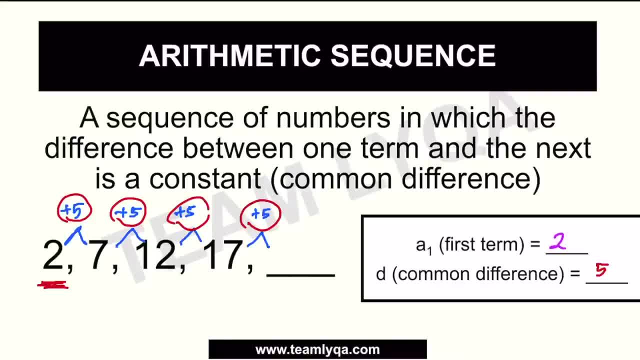 So bisibinan ng common difference ay 5.. Now, kung nawawala yung susunod na term sa sequence na ito, how can we get to that? Titinan lang natin yung 17,, tapos idadagdag natin yung common difference. 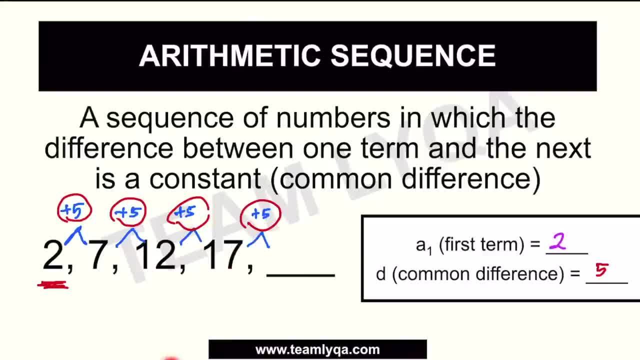 So 17 plus 5,, that would be 22.. So ang ating next Na term would be 22,. okay, Now, that is really easy kung ganito lang yung mga numbers natin, Pero when it comes to your modules or kung paano isasolve ito, 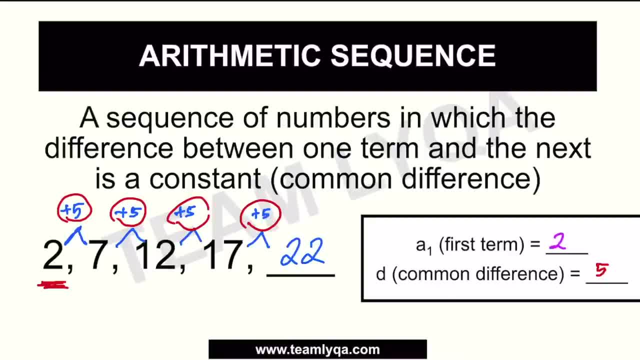 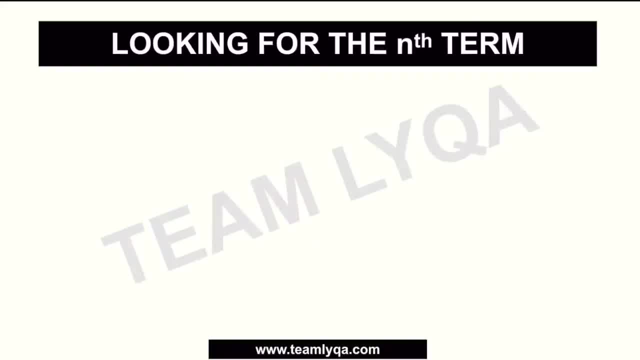 minsan ang hinahanap na term ay yung pang 30 o pang 100. Now, paano natin yung makukuha nang hindi natin kailangan ilista ang lahat Dito na papasok yung hunt natin for the formula that we're going to use. 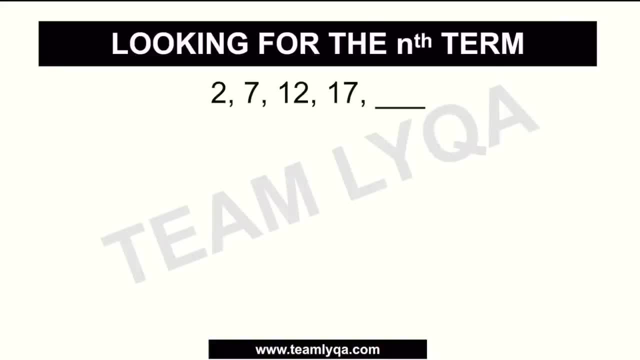 So balikan natin yung information that we had earlier. So try to look for the nth term, Yung pang n na term dun sa sequence na yan. Now, kung titinan natin, kung tatawagin natin yung 2, again, this is the initial term. 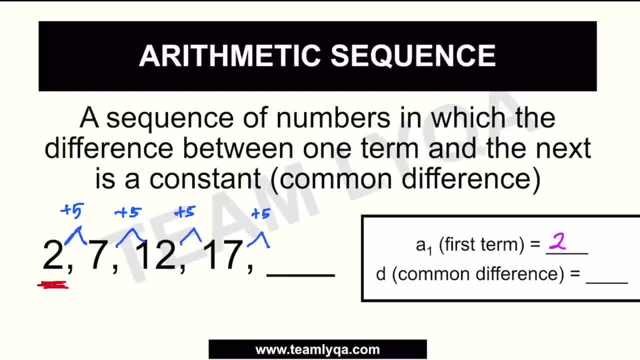 siya dito. Now why is it important? Kasi mamaya sa formula dapat automatic sa atin yung pag-spot common difference, Yun yung constant na pinagkaiba ng mga numbers na yan. Sa case na ito, that is plus 5.. 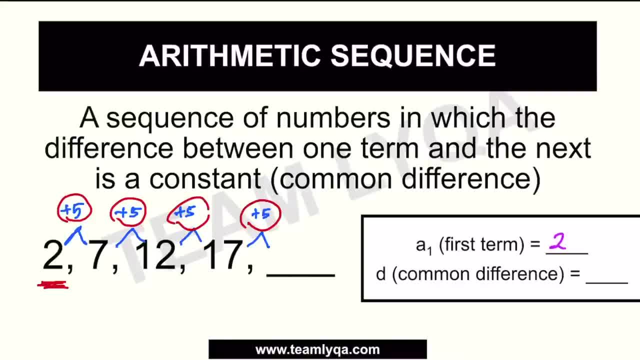 Again pare-pareho. sila So bisibinan ng common difference ay 5.. Now, kung namawala yung susunod na term sa sequence na ito, how can we get to that? Titinan lang natin yung 17,, tapos idadagdag natin yung. 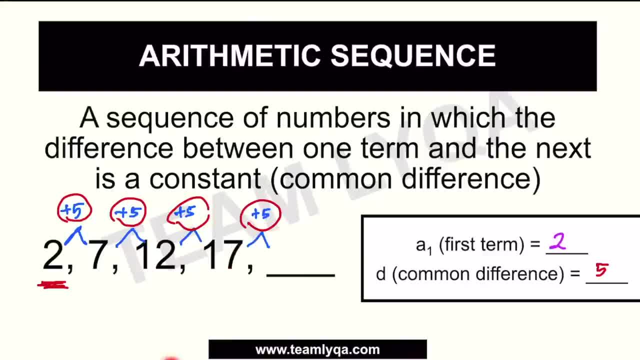 common difference. So 17 plus 5,, that would be 22.. next na term would be 22,. okay, Now, that is really easy kung ganito lang yung mga numbers natin, Pero when it comes to your modules or kung paano isosolve ito, 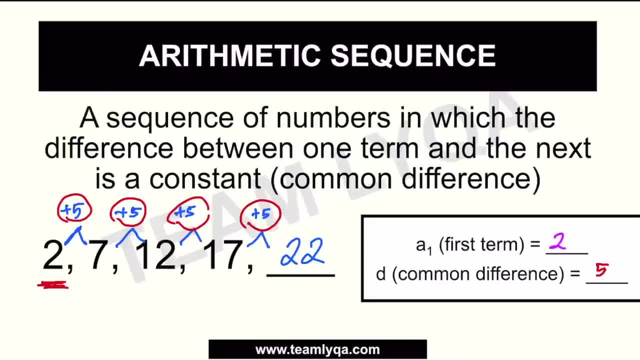 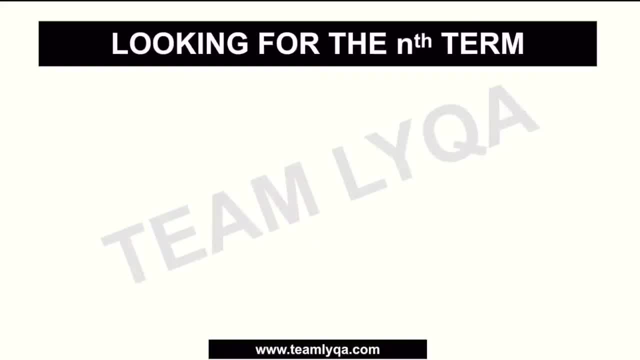 minsan ang hinahanap na term ay yung pang 30 o pang 100. Now, paano natin yun makukuha nang hindi natin kailangan ilista ang lahat. Dito na papasok yung hunt natin for the formula that we're going to use. 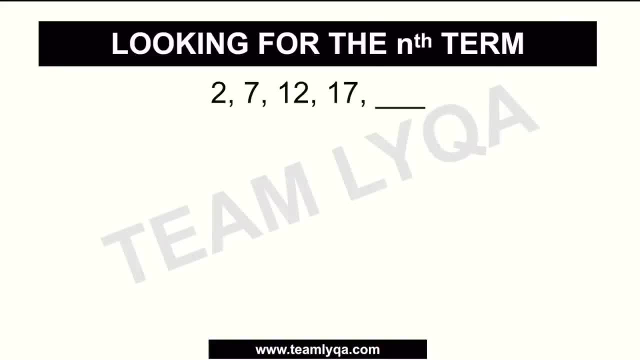 So balikan natin yung information that we had earlier. So try to look for the nth term, Yung pang n na term dun sa sequence na yan. Now, kung titinan natin, kung tatawagin natin yung 2, again, this is the initial term. 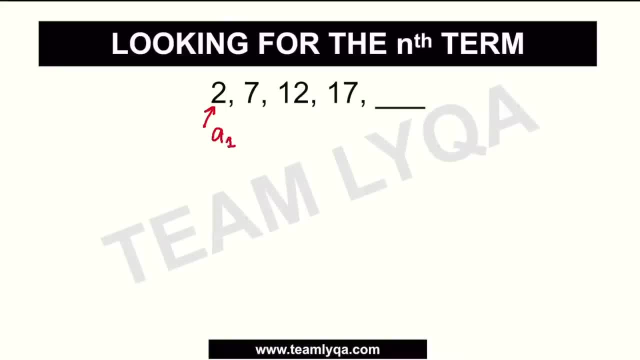 At tatawagin natin syang a sub 1, as in the first term dun sa sequence natin. Tapos, sabi natin di ba yung kanyang pinagkaiba, ang kanyang common difference ay 5.. 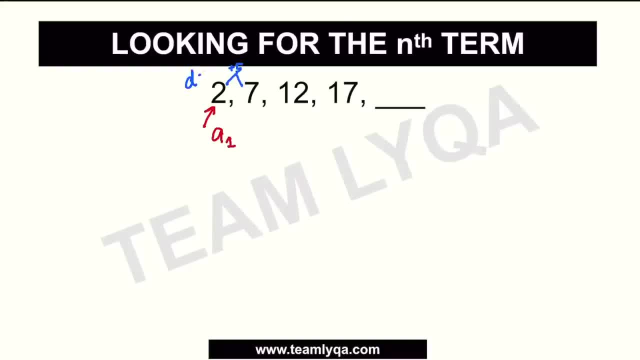 Okay, So that would be our d Tapos, kung titinan natin yung ibang mga numbers, yun yung pwesto nila dun sa sequence. Now, kung ilista natin yan, you would find a pattern which is this: 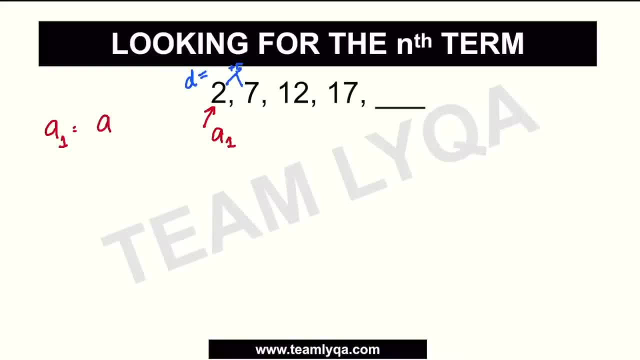 Ang a sub 1,, of course, is equal to a sub 1.. a sub 2,, in this case, ang a sub 2, is 7.. Okay, That is equal to the a sub 1,, which is 2, plus yung difference, which is 5.. 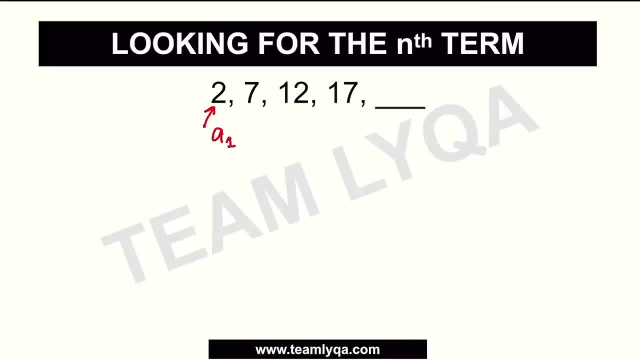 at tatawagin natin syang a sub 1, as in the first term dun sa sequence natin. tapos sabi natin: di ba yung kanyang pinagkaiba, ang kanyang common difference ay 5, okay. 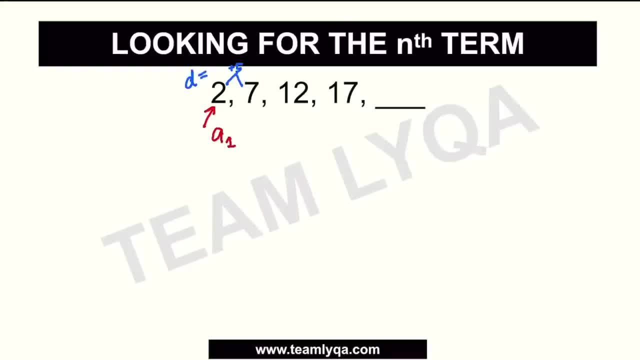 So that would be our d Okay. Tapos, kung titinan natin yung ibang Ibang mga numbers, yun yung pwesto nila dun sa sequence. Now, kung ilista natin yan, you would find a pattern which is this: 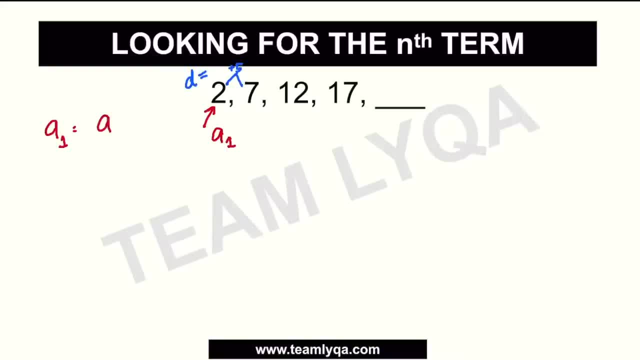 Ang a sub 1,, of course, is equal to a sub 1.. a sub 2,, in this case, ang a sub 2 is 7,. okay, That is equal to the a sub 1,, which is 2, plus yung difference, which is 5.. 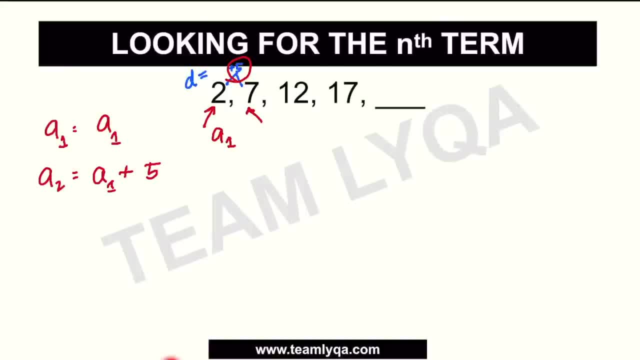 Okay. So I think naiintindihan naman ang lahat. no, Again, bakit naging ganito? Kasi 7 is equal to 2 plus 5, which is the d. Okay, Now, kung hindi natin isusulat sya as 5, at tatawagin natin syang d, okay lang din yun. 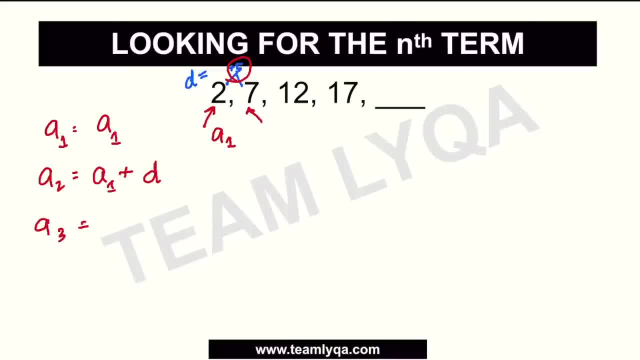 tingnan naman natin yung a sub 3.. Now, if you're going to look at a sub 3 in terms nung a sub 1 and a sub 2, it's basically This 7, or yung a sub 2, plus another 5.. 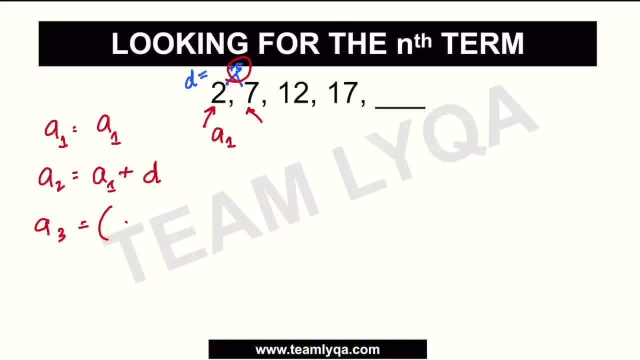 Or itong number na ito, a sub 1 plus d plus another d Diba, Kasi this is now 7 plus 5, which is going to give us 12.. Now this goes on and on sa kung pang ilang term yan. 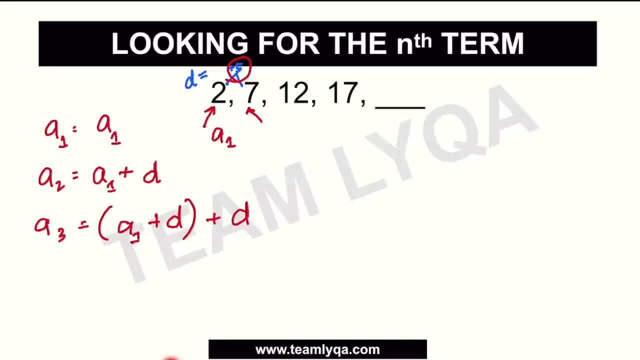 Pero ang pinagkain, Ang pinagkain na iba niya talaga is the number ng mga d na idadagdag natin. Now, bakit ganun? Kasi kung titinan natin yung a sub 4, this is basically a sub 1 plus d plus another d plus another d. 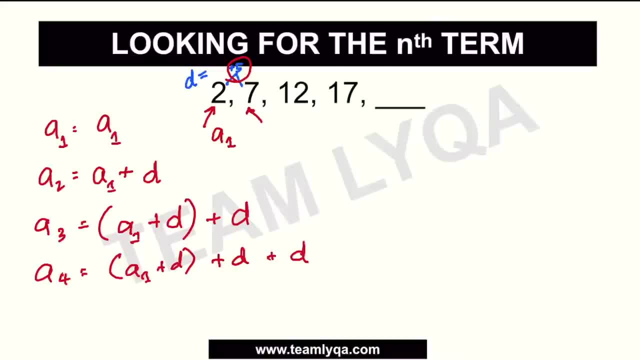 At kung i-group ko yan pagsasamah-samahin natin yung mga d, we can actually write this as a sub: 1 plus 3d. Now tingnan natin kung ano tong 3 na ito. 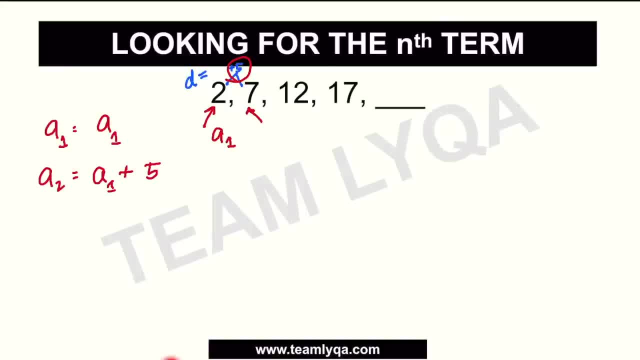 Okay. So I think naiintindihan naman ang lahat. no, Again, bakit naging ganito? Kasi 7 is equal to 2 plus 5, which is the d. Okay, Now, kung hindi natin isusulat sya as 5, at tatawagin natin syang d, okay lang din yun. 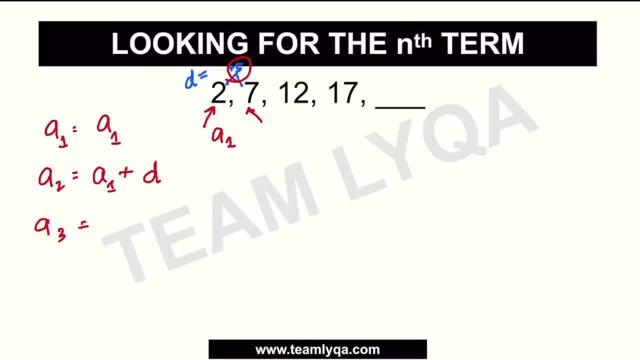 Tingnan naman natin yung a sub 3.. Now, if you're going to look at a sub 3 in terms ng a sub 1 and a sub 2, it's basically this 7, or yung a sub 2, plus another 5.. 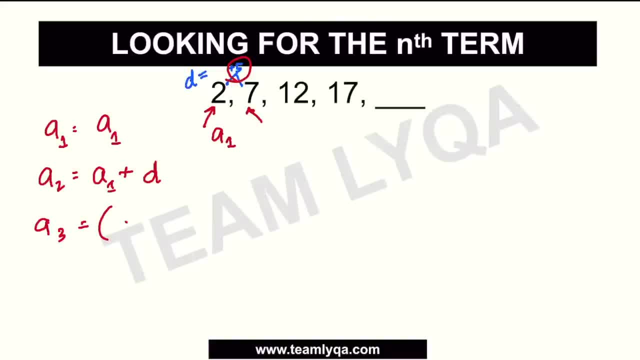 Or itong number na ito, a sub 1 plus d plus another d Diba, Kasi this is now 7 plus 5, which is going to give us 12.. Now this goes on and on sa kung pang ilang term yan. 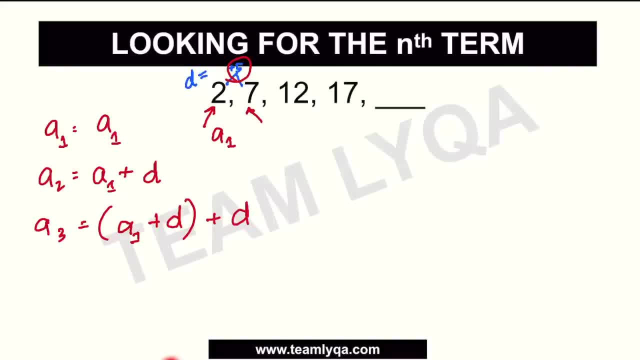 Okay. Ang pinagkaiba niya talaga is the number ng mga d na idadagdag natin. Now, bakit ganon? Kasi, kung titinan natin yung a sub 4, this is basically a sub 1 plus d plus another d plus another d. 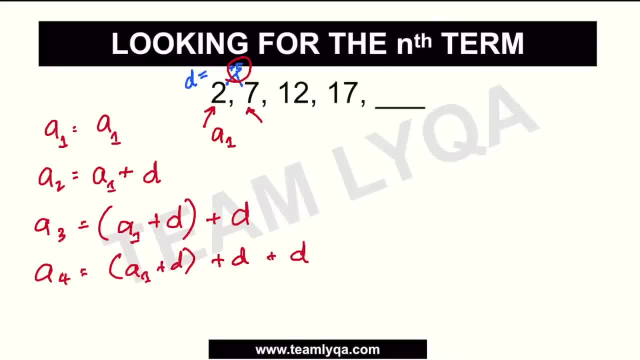 At kung i-group ko yan pagsasamah-samahin natin yung mga d, we can actually write this as a sub: 1 plus 3d. Now tingnan natin kung ano tong 3 na ito. 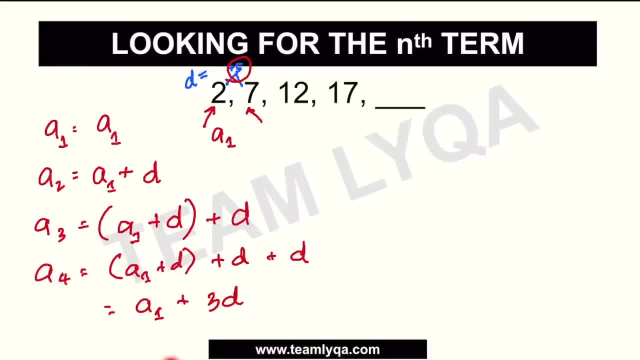 In reference doon sa order or doon sa placement nung nawawalang term Diba, ang 3 is basically 4 minus 1? Now that would give us a clue doon sa ating gagamitin formula. What do I mean by that? 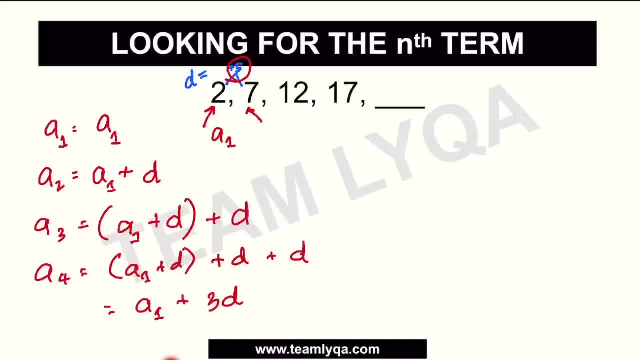 Kasi yung 3 is basically 4 minus 1.. Now isusulat ko siya as that ha Tingnan nyo to, This is basically a sub 1 plus yung number na sa ilalim or yung position niya. 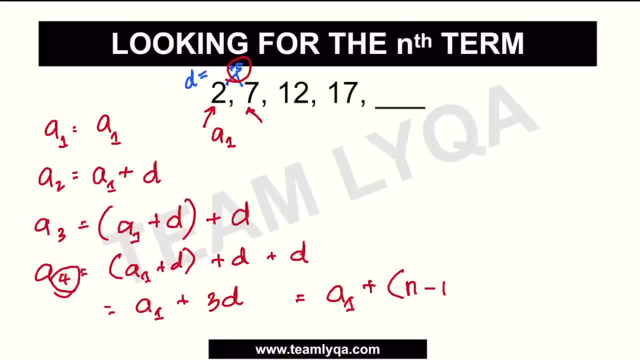 So that is, n Tawagin natin siyang n Minus 1 multiplied by d. Now, the best way for us to check if this works is to see if yung susunod nating term, in this case this right here, is a sub 5,. 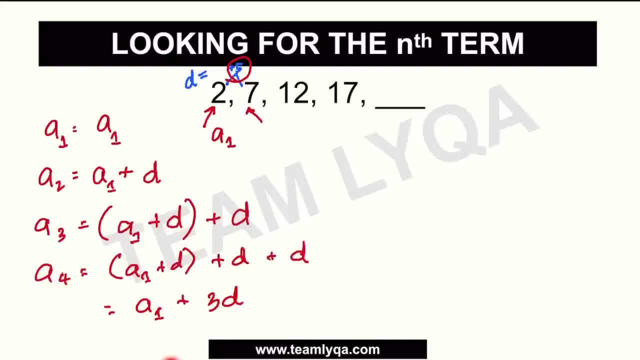 In reference doon sa order or doon sa placement nung nawawalang term Diba, ang 3 is basically 4 minus 1? Now that would give us a clue doon sa ating gagamitin formula. What do I mean by that? 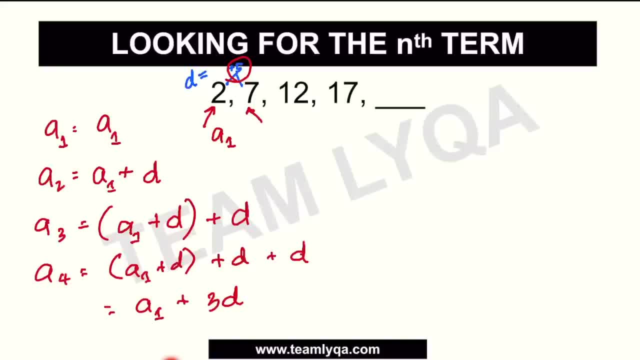 Kasi yung 3 is basically 4 minus 1.. Now isusulat ko siya as that ha Tingnan nyo to, This is basically a sub 1 plus yung number, yung number nasa ilalim or yung position niya. 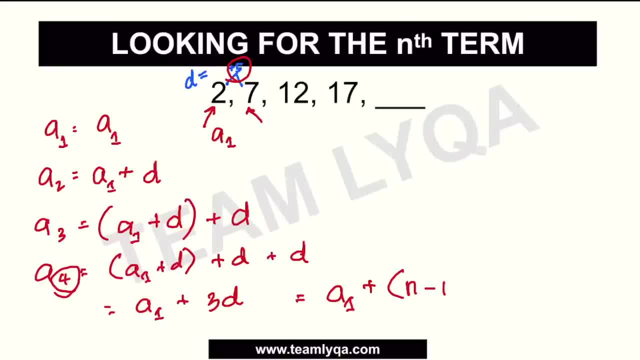 So that is, n Tawagin natin siyang n minus 1 multiplied by d. Now the best way for us to check if this works is to see if yung susunod nating term, in this case this right here, is a sub 5,. 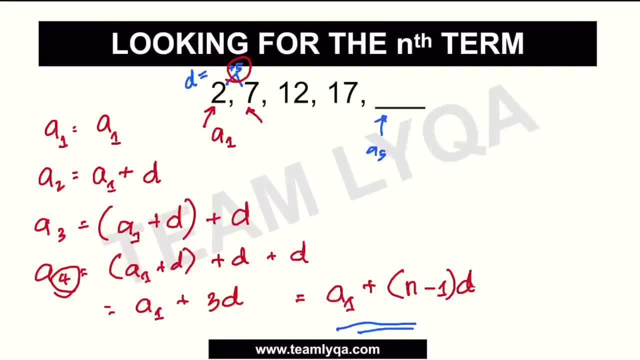 will be correct kung gagamitin natin yung formula na ito. Okay, Now tingnan natin. ha, yung information natin. Ang hinahanap natin hindi na n's term. We're looking for the fifth term doon sa ating sequence. 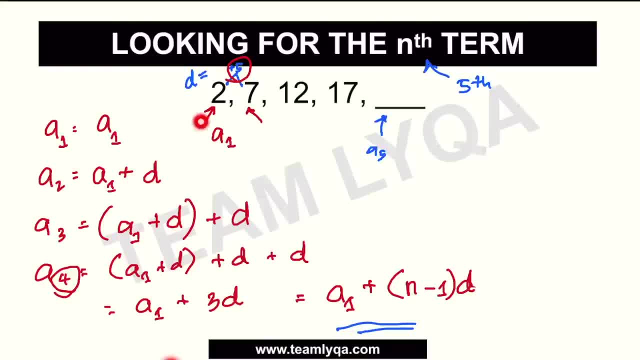 Now to substitute yung ating mga given a sub, 1 would be the first or initial term, So that would be 2.. Tapos plus yung parentheses natin, Tapos n minus 1.. Again, ang n natin ay 5.. 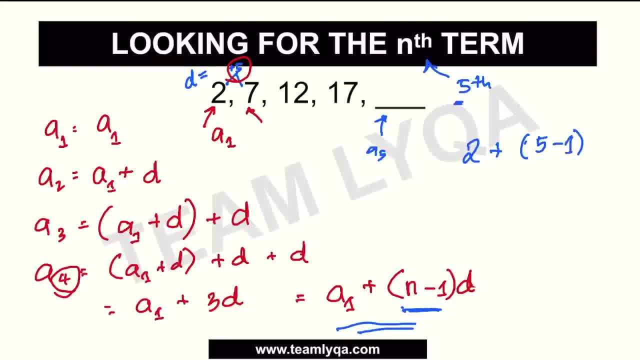 So that would be 5 minus 1 multiplied by the d, which is 5.. Now, kung isosolve natin ito again, we're looking for the fifth term, a sub 5, or the fifth term is equal to 2 plus the quantity 5 minus 1 is 4 times 5,. 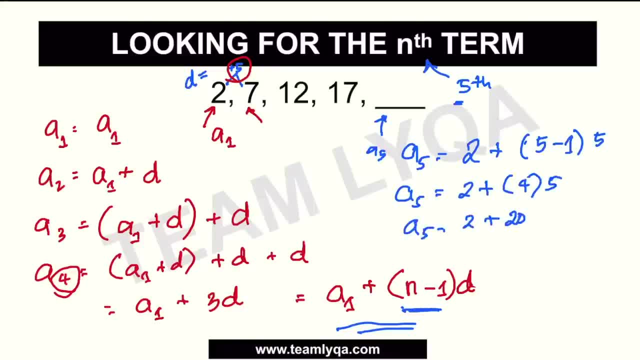 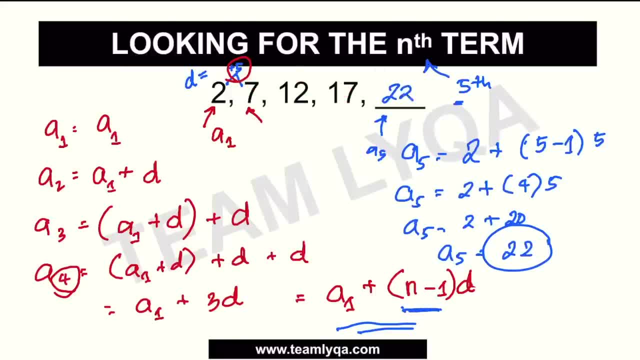 17 plus 5, ba 22?? Now ang sagot, dyan ay oo. So ibig sabihin, tama tayo dito. So doon natin nakuha yung ating formula, which is going to be this: 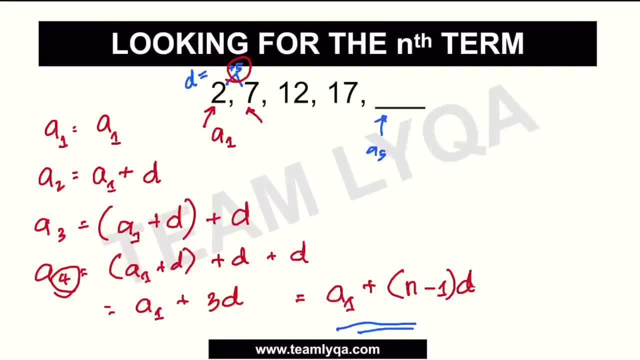 will be correct kung gagamitin natin yung formula na ito. Okay, Now tingnan natin. ha yung information natin Ang hinahanap natin, hindi na n Next term. we're looking for the fifth term doon sa ating sequence. 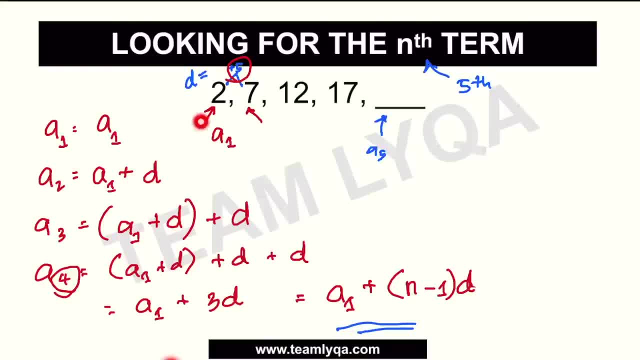 Now to substitute yung ating mga given a sub, 1 would be the first or initial term, So that would be 2.. Tapos plus yung parentheses natin, Tapos n minus 1.. Again, ang n natin ay 5.. 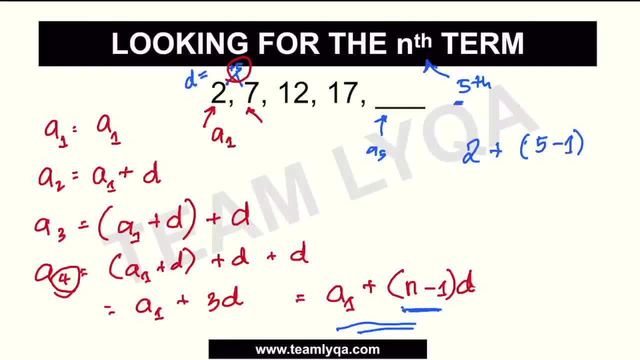 So that would be 5 minus 1 multiplied by the d, which is 5.. Now, kung isosolve natin ito again, we're looking for the fifth term, a sub 5, or the fifth term is equal to 2 plus the quantity 5 minus 1 is 4 times 5. 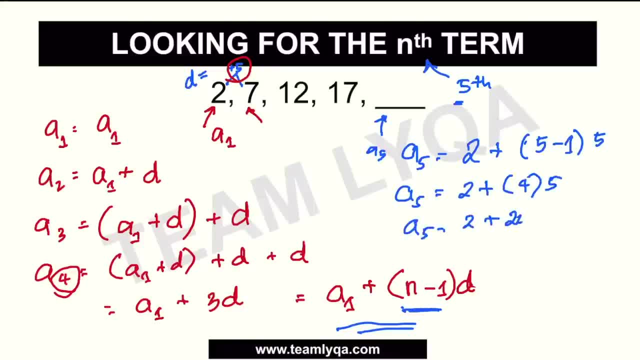 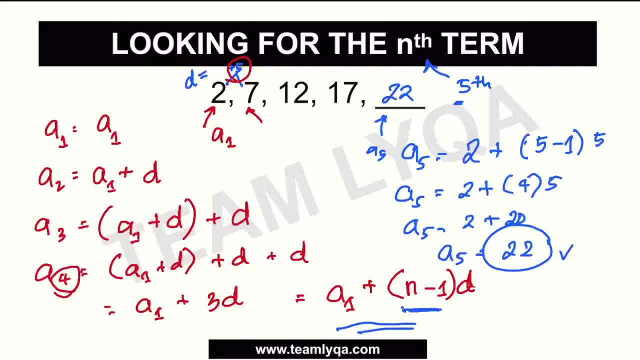 Now ang sagot natin. So ibig sabihin, tama tayo dito. So doon natin nakuha yung ating formula, which is going to be this: The nth term is equal to a sub 1 plus the quantity n minus 1 times d. 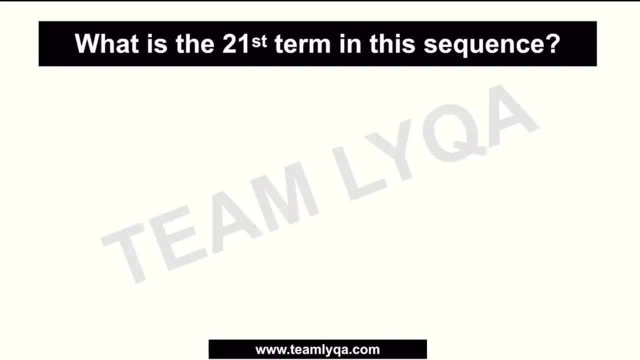 Okay, Now paano natin gagamitin yun, Kung ganito yung tanong sabi: what is the 21st term in this sequence? Tapos meron tayong sequence na ganito: 3, 9.. 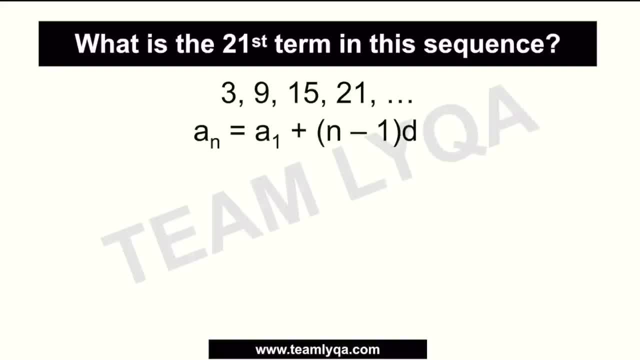 15 and 21.. Using the formula, hindi na natin kailangan bilangin yung blanks Diba. Kasi imagine kung ilang blank yung lalagay mo diba Hanggang maka 21 ka. 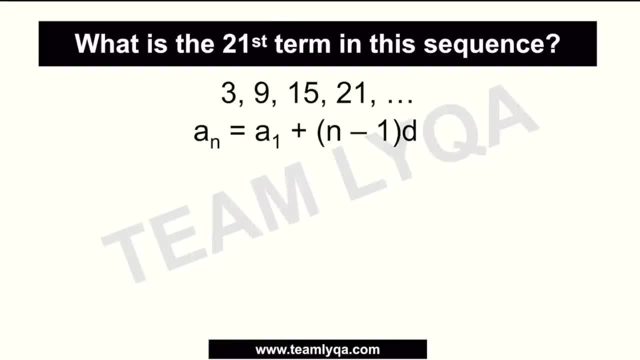 Maka hindi ka na matapos. So ang gagamitin natin instead would be to use the formula and just substitute yung mga given dito sa sequence na ito. Now i-rewrite lang natin a sub n. in this case, ang hinahanap natin is the 21st term. 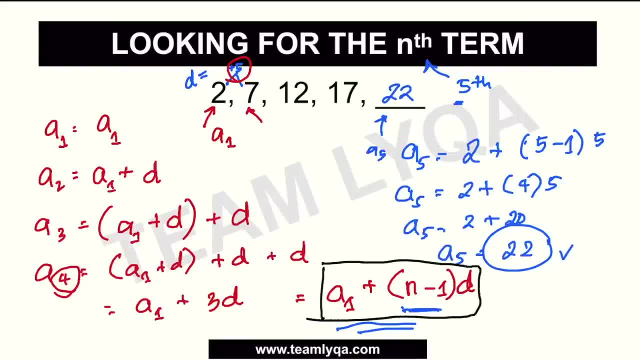 The n'th term is equal to a sub 1 plus the quantity n minus 1 times d. Okay, Now paano natin gagamitin yun Kung ganito yung tanong sabi: what is the 21st term in this sequence? 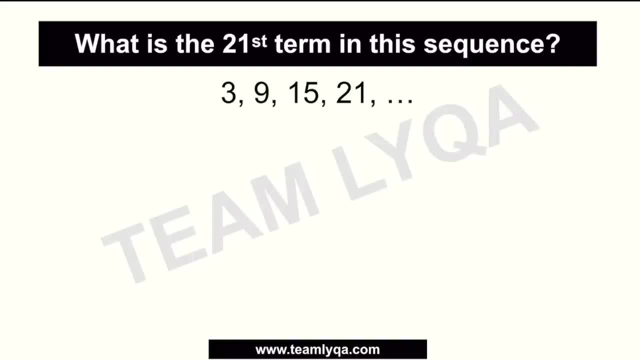 Tapos meron tayong sequence na ganito: 3,, 9,, 15, and 21.. Using the formula, hindi na natin kailangan bilangin yung blanks Diba, Kasi imagine kung ilang blank yung lalagay mo diba. 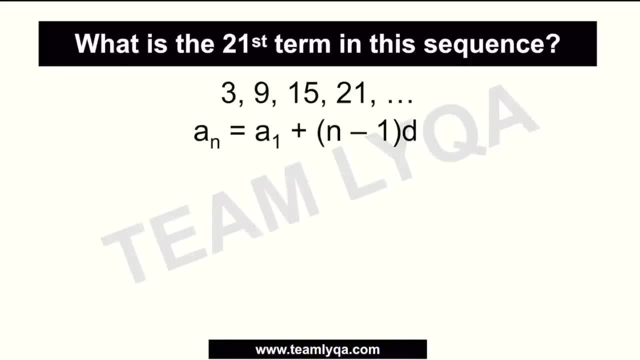 Hanggang maka 21 ka Maka. hindi ka na matapos. So ang gagamitin natin instead would be to use the formula and just substitute yung mga given dito sa sequence na ito. Now i-rewrite lang natin. 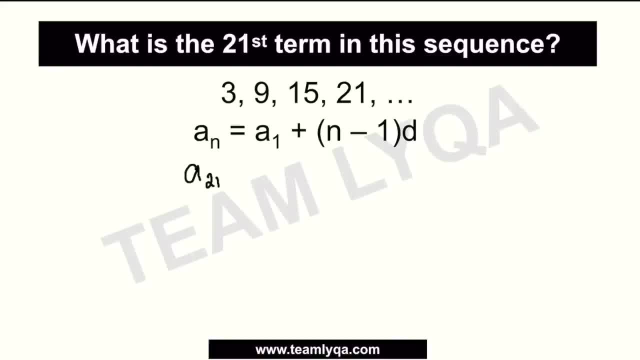 a sub n. in this case, ang hinahanap natin is the 21st term, So yung n is 21. is equal to a sub 1, or the 1st term, So that is actually 3.. 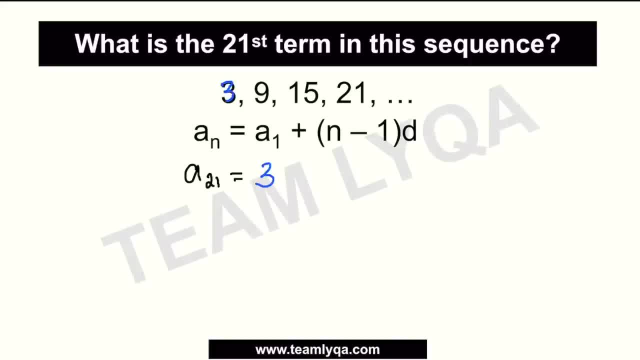 So lagay natin 3.. Tapos, plus the quantity na n, Again ang n would be itong 21st term in the sequence. So yun yung nahanap, 21.. Lagay lang natin dyan. 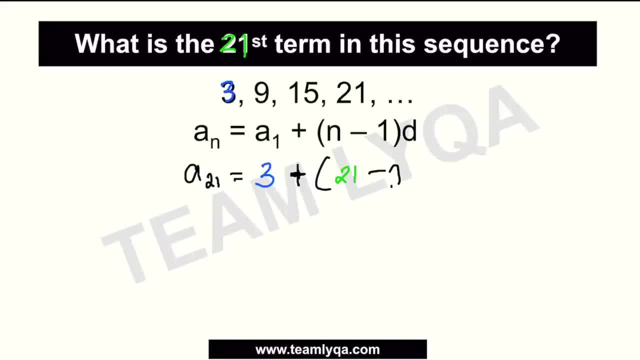 21. Minus 1. Yung 1 is a constant, So hindi na natin babaguhin yan Laging 1 yan Minus 1. Times the d Or the common difference. Now, ano bang common difference nito? 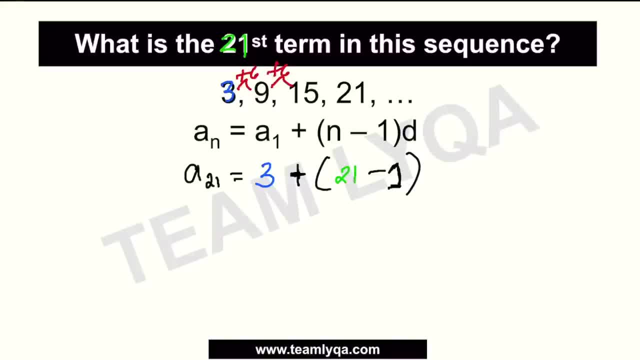 3 plus 6 is 9.. 9 plus 6 is 15.. 15 plus 6 is 21.. So ang common difference ay 6.. Okay, now that we have all of the information, subukan na natin isolve. 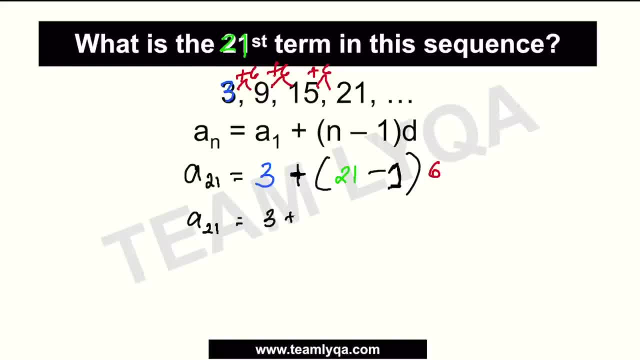 The 21st term is equal to 3 plus 21 minus 1 is 20 times 6.. So a the 21st term is equal to 3 plus 20 times 6, which is 106.. So a the 21st term is equal to 3 plus 20 times 6,, which is 106. 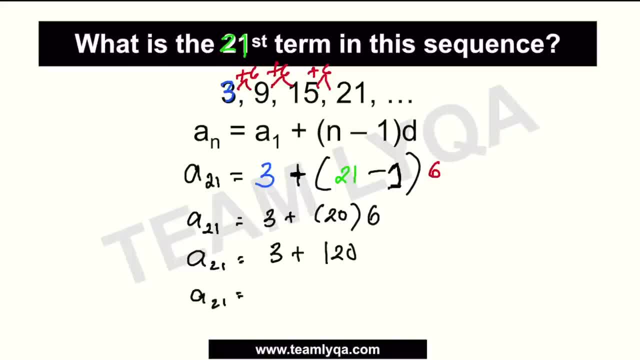 So a sub 21 is 123.. So the answer is 123, ang 21st term in that sequence. So, using the formula, hindi ko na kailangan isa-isahin. mag add ng 6 ng paulit-ulit. 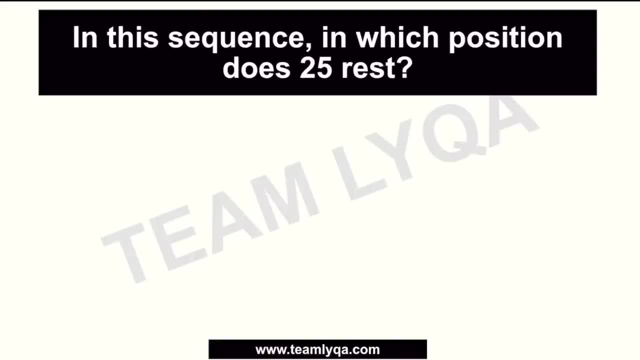 Now, paano naman kung ang nawawala ay yung position, Basically the end Sabe in this sequence, in which position does 25 rest, rest, Now again pwede kong lagyan ng mga blank? 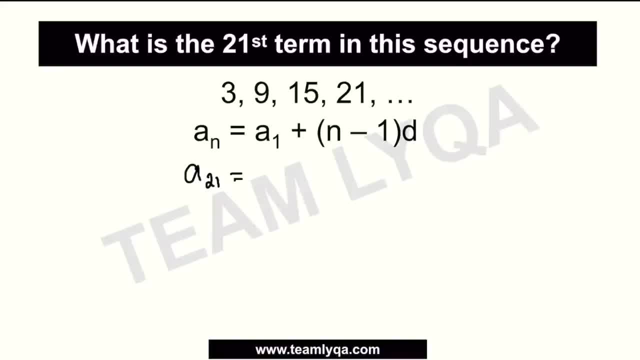 So yung n is 21.. It's equal to a sub 1, or the first term, So that is actually 3.. So lagay natin 3.. Tapos plus the quantity na n, Again ang n would be itong 21st term in the sequence. 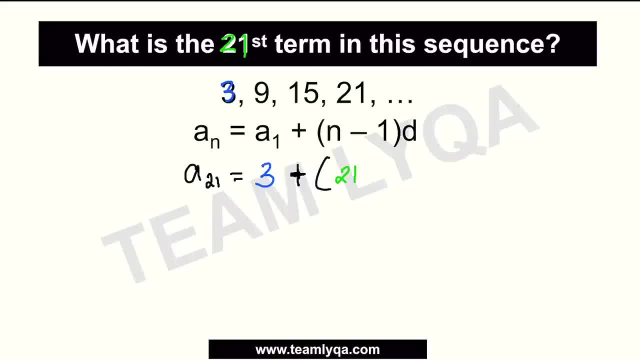 So yun yung nahanap: 21. Lagay lang natin dyan 21. Minus 1. Yung 1 is a constant, So hindi na natin babaguhin yan. Laging 1 yan. 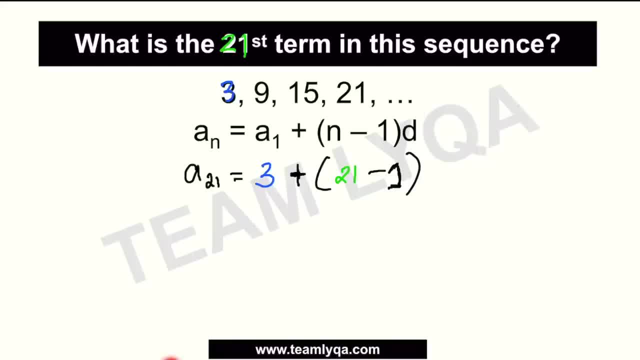 Minus 1.. Times the d or the common difference. Now, ano bang common difference nito: 3 plus 6 is 9.. 9 plus 6 is 15.. 15 plus 6 is 21.. So ang common difference ay 6.. 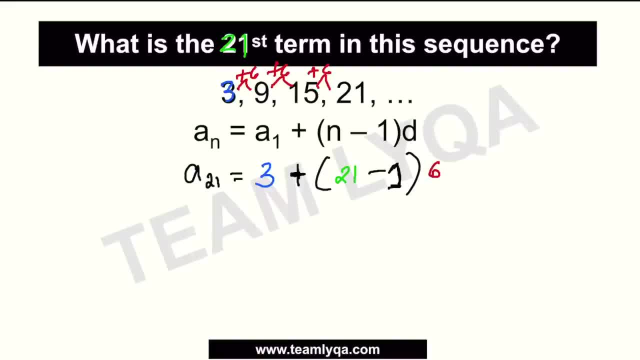 Okay Now, now that we have all of the information, subukan na natin isolve. The 21st term is equal to 3 plus 21 minus 1 is 20.. Times 6. So a The 21st term is equal to 3 plus 20 times 6,, which is 120. 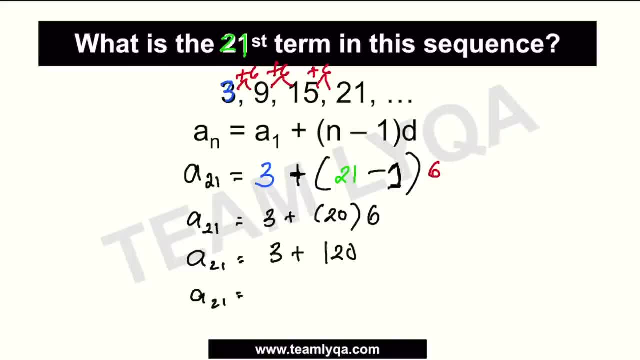 120.. A sub 21, that is 123.. So the answer is 123, ang 21st term in that sequence. Okay, So, again using the formula, hindi ko na kailangan isa-isahin na mag-add ng 6 ng paulit-ulit. 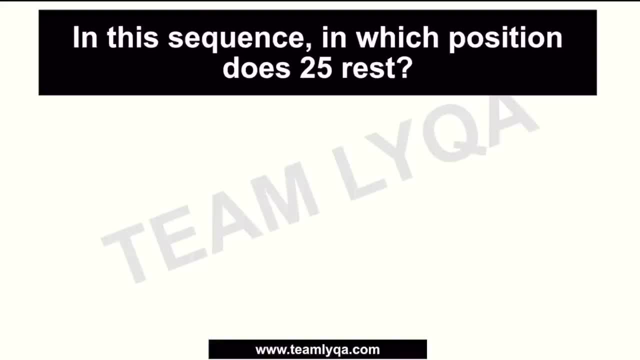 Now, paano naman kung ang nawawala ay yung position, Basically the end Sabi in this sequence. in which position does 25 rest? Now again pwede kong lagyan ng mga blank dyan, ang paulit-ulit hanggang makakarating ako dun sa 25.. 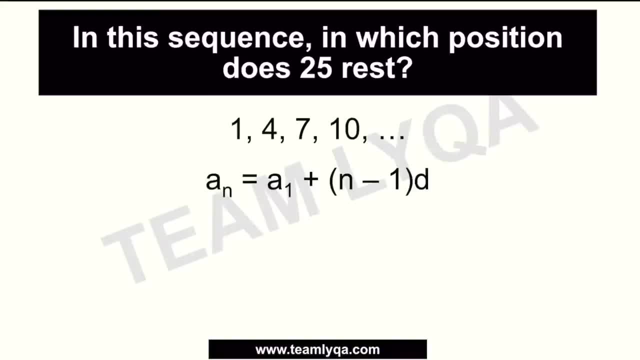 Or I could just use the formula. Now, using the formula, isa-substitute lang natin yung mga nakita na natin dito sa problem natin. Now, yung 25 is actually yung a sub n Hindi lang natin alam kung ano yung n. 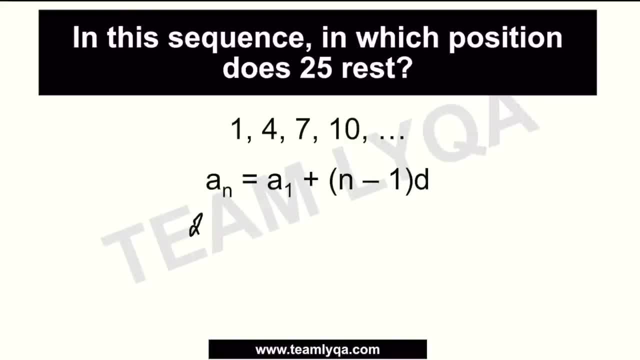 So ibig sabihin, nun, dito sa left side ilalagay natin yung 25.. Equal, siya dun sa. Ang initial term is 1. Plus yung n which is missing. So again, we'll keep it at n na lang. 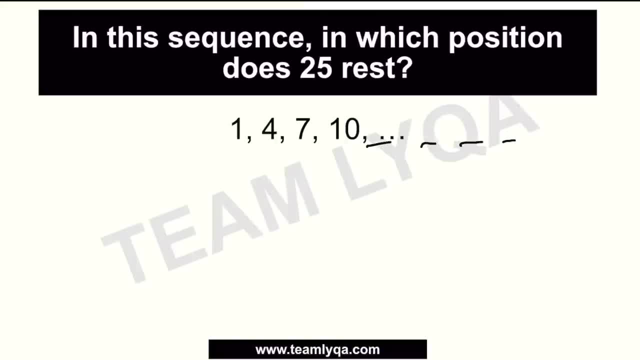 dyan ang paulit-ulit hanggang makakarating ako dun sa 25, or I could just use the formula Now. using the formula, isasubstitute lang natin yung mga nakita na natin dito. 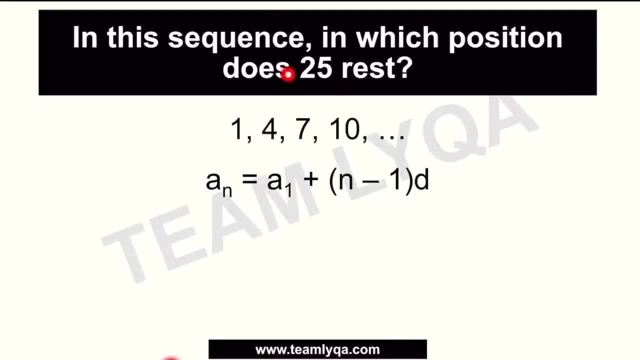 sa problem natin Now, yung 25 is actually yung a sub n. Hindi lang natin alam kung ano yung n. So ibig sabihin, nun dito sa left side ilalagay natin yung. 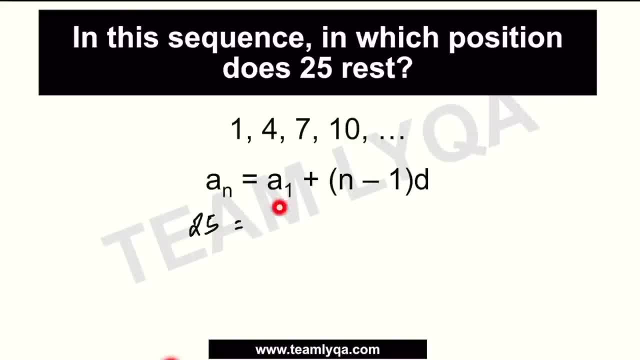 25. Equal, sya dun sa, ang initial term is 1, plus yung n which is missing. So again, we'll keep it at n na lang, Minus 1 times the d or the common difference. Now ang common difference dito. 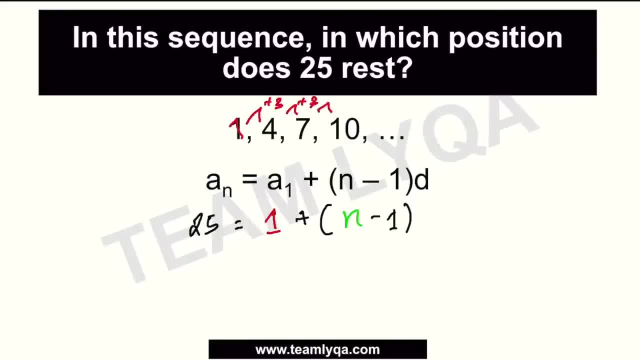 you have plus 3,, plus 3, and plus 3.. So this will be 3.. Now all we have to do is to solve for n. So ang una natin gagawin is to move this here. So 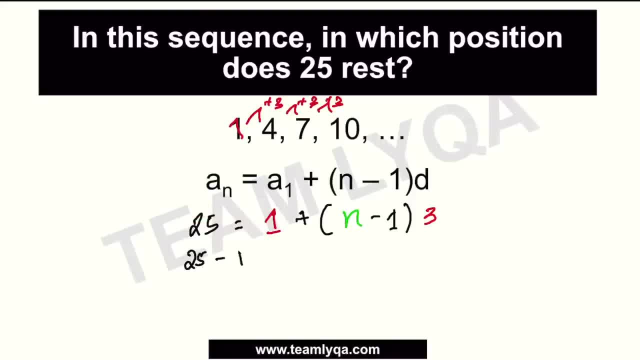 ang gagawin natin: 25 minus 1 is equal to now you have n minus 1, yung quantity na yan times 3. So pwede natin sya i-distribute dito, Okay, So this will be 3. 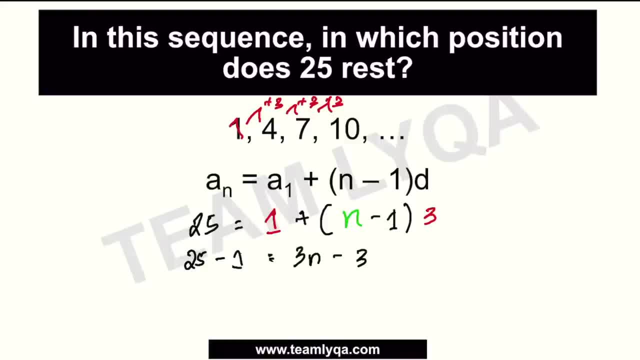 n minus 3.. Okay, now 24 na ito. tapos itong 3 na ito pwede natin i-group or i-transpose, natin dyan, I-dipat lang natin yung negative 3, magiging plus 3 sya. 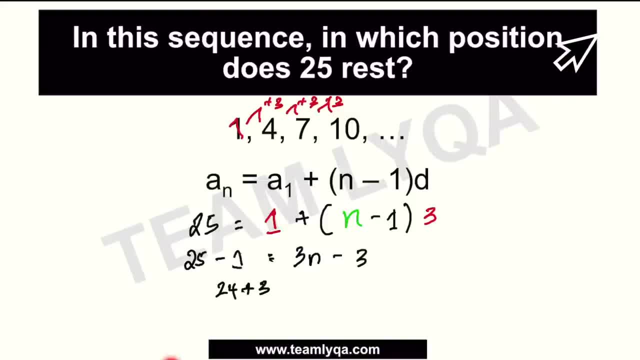 This is just basically parang solving for x ha. Kung hindi nyo pa napapanood yung video na yun, i-link ko lang lang din dito sa taas. It's equal to 3n Now, 24 plus 3. 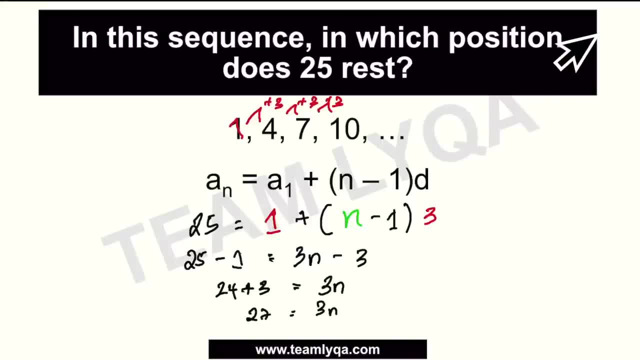 is 27.. It's equal to 3n. I-divide natin both sides by 3.. Makakancel ito, maiiwan yung n And 27 divided by 3 is 9.. So ibig sabihin nun, n. 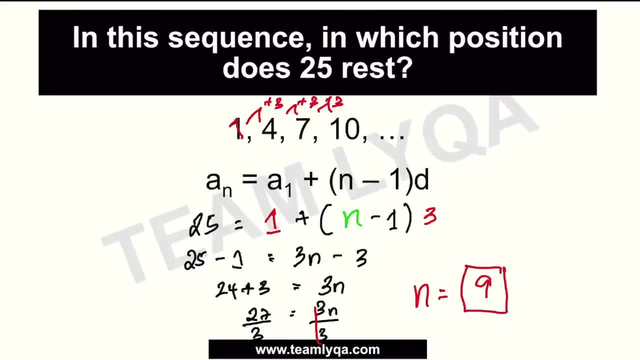 is equal to 9.. Ibig sabihin, ang number na 25 is the 9th term in the sequence. Now, if you want to check, you can fill in the blacks. So this is 1,, 2,, 3,. 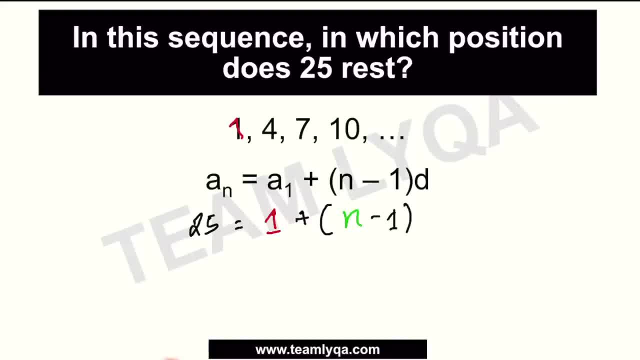 Minus 1 times the d or the common difference. Now ang common difference dito, you have plus 3,, plus 3, and plus 3.. So this will be 3.. Now all we have to do is to solve for n. 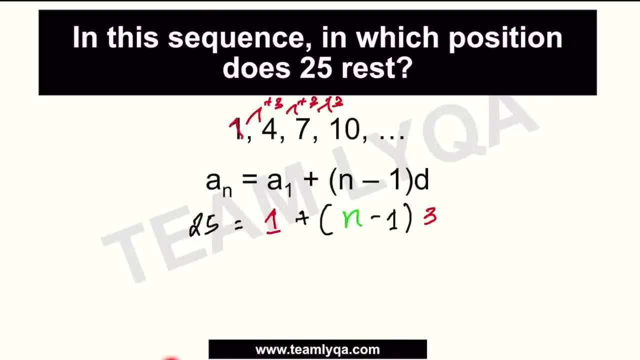 So ang una natin gagawin is to move this here. So ang gagawin natin: Yung 25 minus 1 is equal to, Now you have n minus 1, yung quantity na yan times 3.. 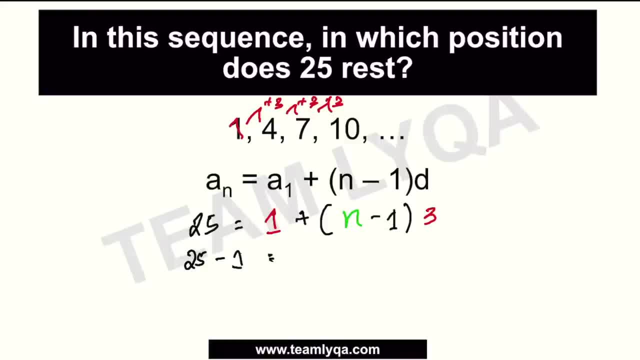 So pwede natin siya i-distribute dito. Okay, So this will be 3n minus 3.. Okay, now 24 na ito. Tapos itong 3 na ito pwede natin i-group or i-transpose natin dyan. 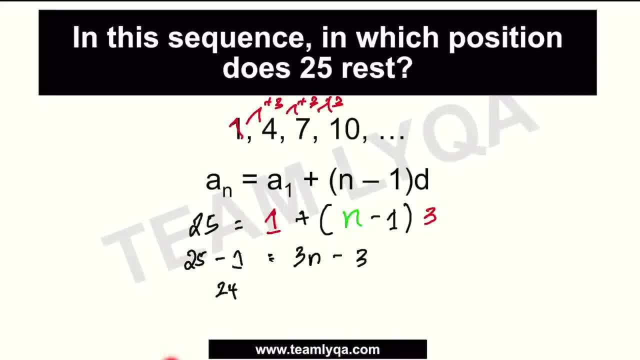 I-dipat lang natin yung negative 3, magiging plus 3 siya. This is just basic, Basically parang solving for x ha. Kung hindi nyo pa napapanood yung video na yun, i-link ko lang lang din dito sa taas. 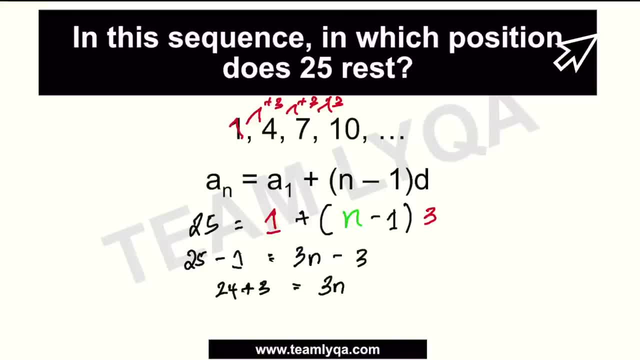 It's equal to 3n. Now, 24 plus 3 is 27.. It's equal to 3n. I-divide natin both sides by 3.. Makakansal, ito maiiwan yung n. 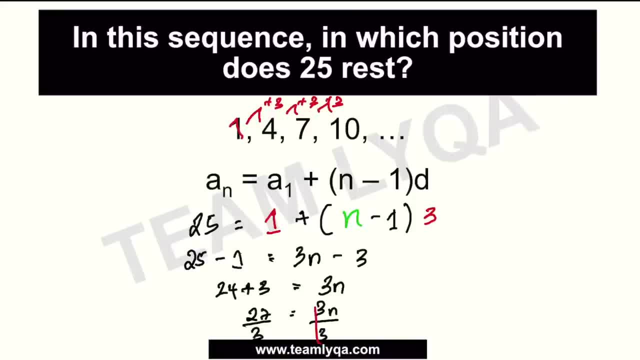 And 27 divided by 3 is 9.. So ibig sabihin nun n is equal to 9.. Ibig sabihin ang number na 25 is: It's the 9th term in the sequence. 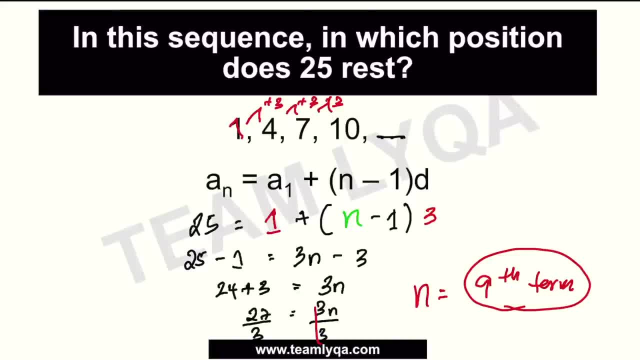 Now, if you want to check, you can fill in the blanks. So this is 1,, 2,, 3,, 4,, 5,, 6,, 7,, 8, and 9.. Again, the difference is 3.. 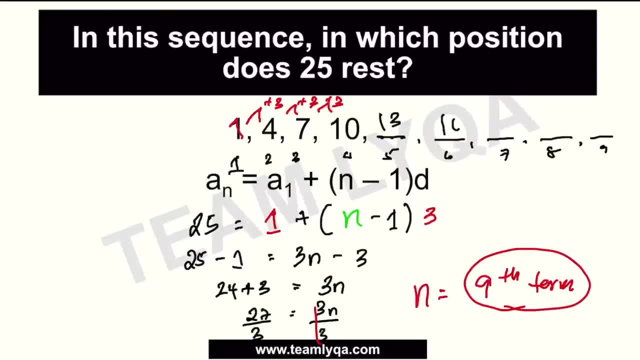 So 10,, 13,, 16,, 19,, 22, and 20.. So tama tayo dyan, It's actually the 9th term. Okay, Now another type of problem that could arise would be something like this: 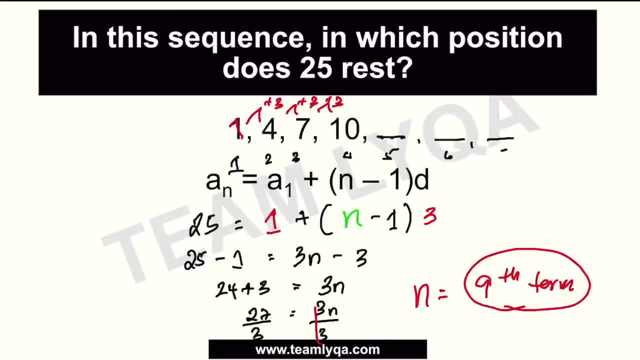 4,, 5,, 6,, 7,, 8, and 9.. Again, the difference is 3.. So 10,, 13,, 16,, 19,, 22, and 20.. So tama tayo, dyan, It's actually the 9th term. 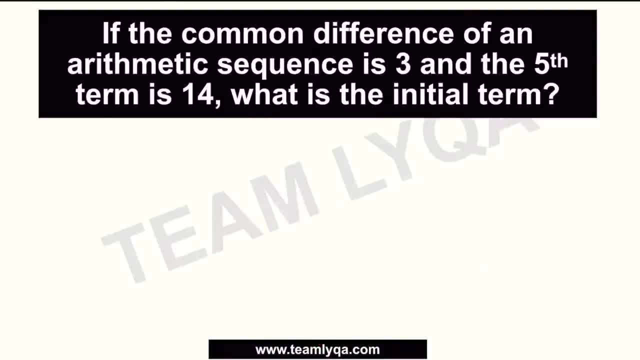 Okay, Now another type of problem that could arise would be something like this: Ang sabi, if the common difference of an arithmetic sequence is 3 and the 5th term is 14, what is the initial term In this case? ang nawawala. 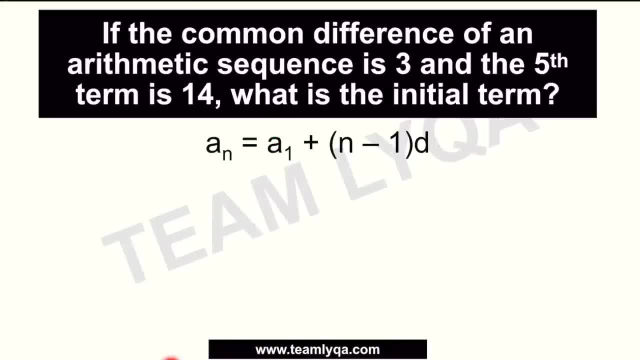 is this yung a sub 1.. So again, all we have to do is to fill in the information. What we have is the 5th term, which is 14.. So sya yung lalagay ko dito sa right side. 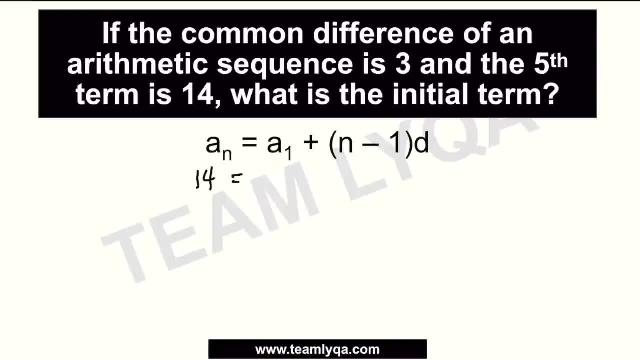 So 14 is equal to again yung a sub 1, hindi pa natin alam, sya yung nawawala a sub 1 plus, and then you have your n. Ang n natin ngayon is: 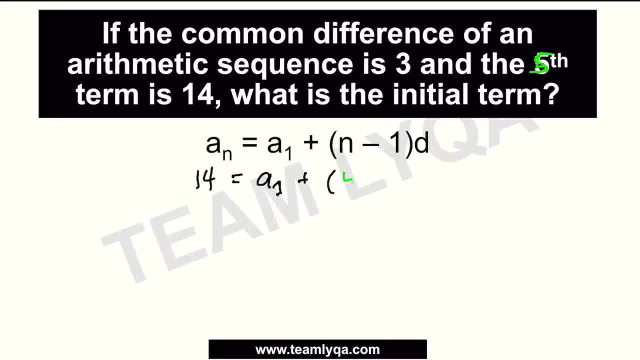 5, kasi 5th term yung 14.. So 5 minus 1 times the d. Now sinabi na lang sya ngayon: Ang common difference ay 3.. So this will be 3.. 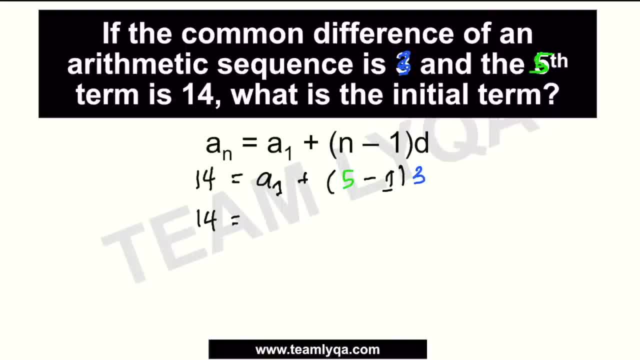 So isosolve lang din natin, following the rules ng finding ng x natin sa algebra. Again, ito ay nahanap lamang sa algebra at hindi sa totoong buhay. a sub 1 plus, and then you have. 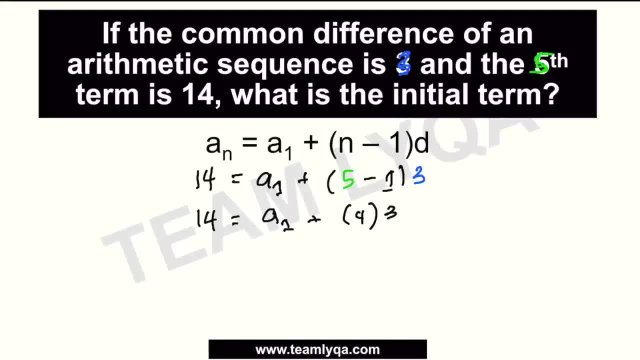 5 minus 1, which is 4 times 3.. 14 is equal to a sub 1 plus 12.. Okay Tapos, kung gusto natin ilipat to sa side na yon, pwede natin parehong i-12 itong. 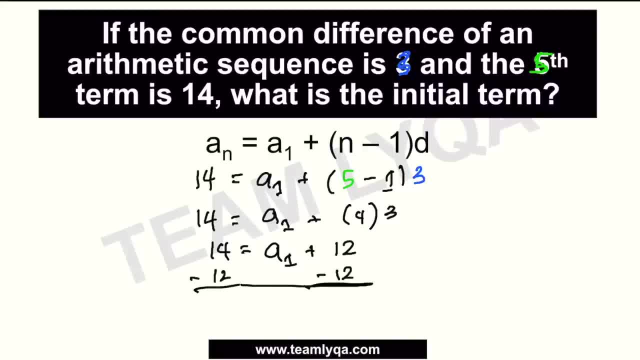 both sides. Okay, So this will be 14 minus 12, or 2 is equal to a sub 1.. Okay, Makakancel, ito kasi positive 12 plus negative 12 is 0.. So ang a sub 1 ay. 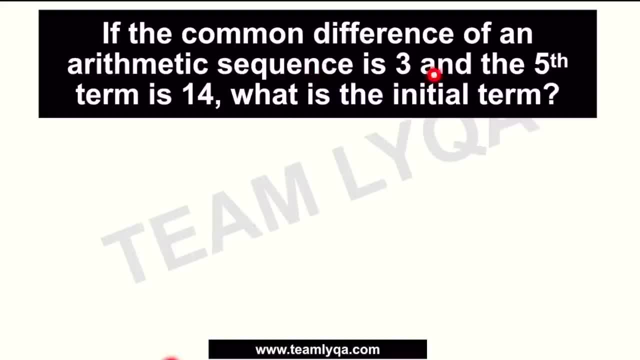 Ang sabi: if the common difference of an arithmetic sequence is 3, and the 5th term is 14,, what is the initial term? In this case, ang nawawala is this, yung a sub 1.. So, again, all we have to do is to fill in the information. 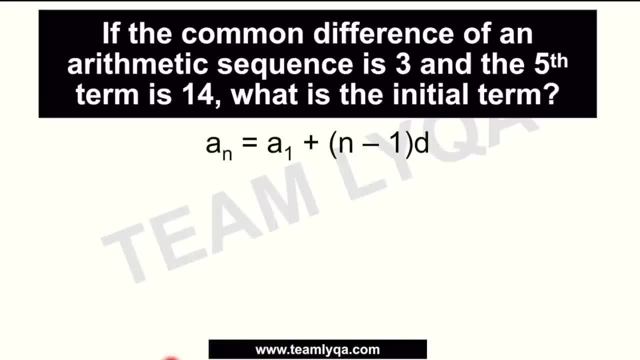 What we have is the 5th term, which is 14.. So sya yung lalagay ko dito sa right side. So 14 is equal to again yung a sub 1, hindi pa natin alam. 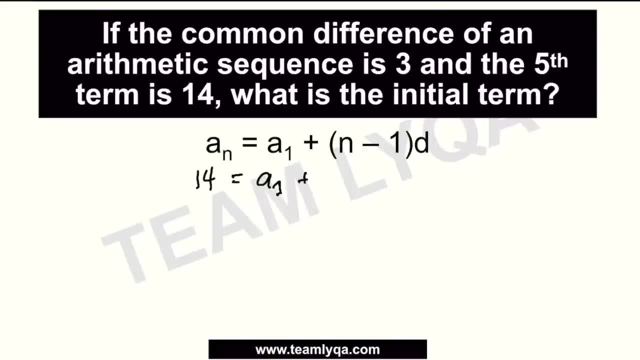 Sya yung nawawala. a sub 1 plus and then you have your n. Ang n natin ngayon is 5,, kasi 5th term yung 14.. So 5 minus 1 times the d. 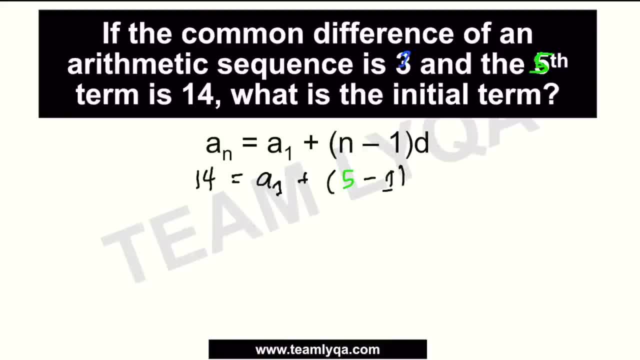 Now sinabi na lang sya: ngayon Ang common difference ay 3.. So this will be 3.. So isosolve lang din natin following the rule. So yung a sub 1 plus ng finding ng x natin sa algebra. 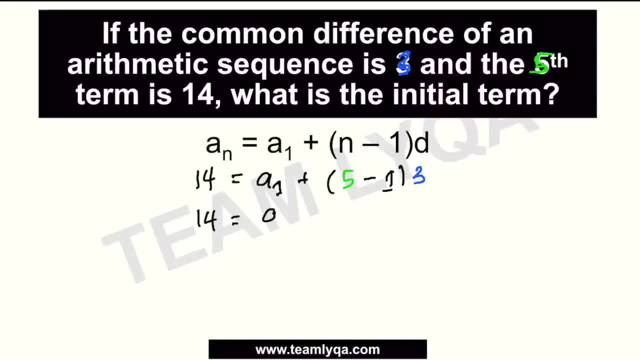 Again, ito ay nahanap lamang sa algebra at hindi sa totoong buhay. a sub 1 plus, and then you have 5 minus 1, which is 4, times 3.. 14 is equal to a sub 1 plus 12.. 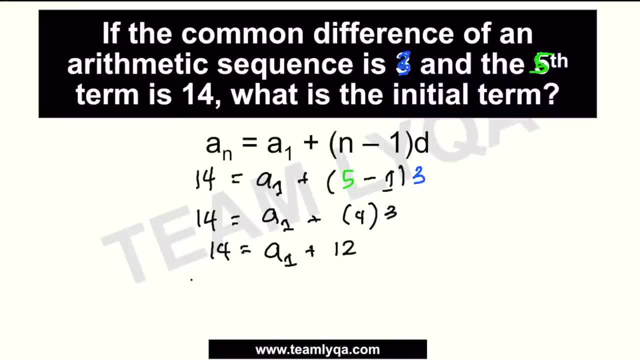 Okay. Tapos, kung gusto natin ilipat ito sa side na yon, pwede natin parehong i-12 itong both sides. Okay, So this will be 14 minus 12 or 2.. 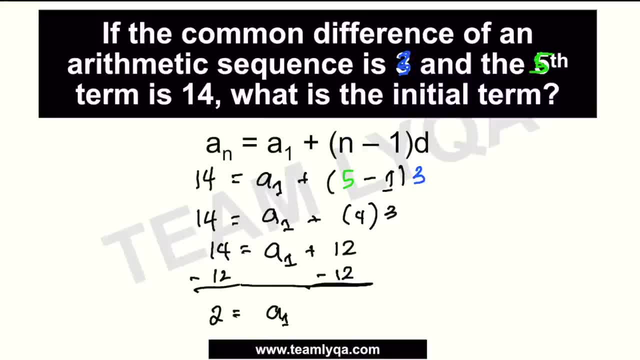 This equals to 12.. This equals to 14 minus 12 or 2.. This is equal to a sub 1.. Okay, Makakancel ito, kasi positive 12 plus negative 12 is 0.. So ang a sub 1 ay 2.. 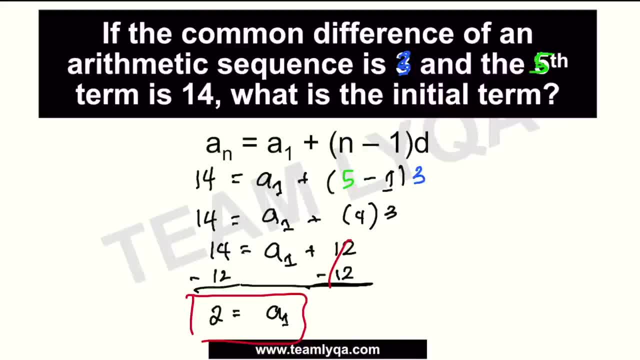 The initial term is 2. And with a common difference of 3,, the 5th term will be 14.. Again, gusto natin i-check kung tama yung pagkakagamit natin. You have 1st term, 2nd, 3rd, 4th and 5th. 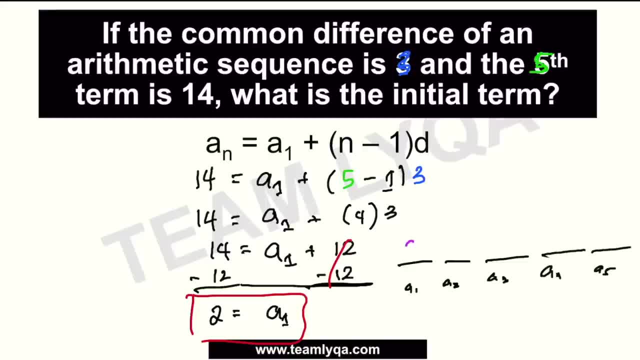 Kung ang ating 1st term ay 2, next would be 5,, 8,, 11, and 14.. So tama tayo dyan. The 5th term is 14 if the initial term is 2, with a common difference of 3.. 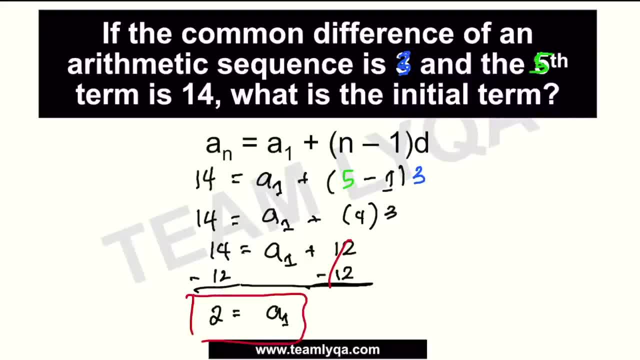 2. The initial term is 2 and with a common difference of 3, the 5th term will be 14.. Again, gusto natin i-check kung tama yung pagkakagamit natin. You have 1st. 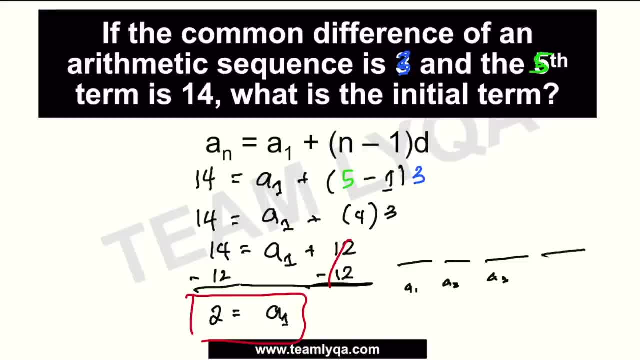 term 2nd, 3rd, 4th and 5th. Kung ang ating 1st term ay 2,, next would be 5,, 8,, 11, and 14.. So tama tayo. 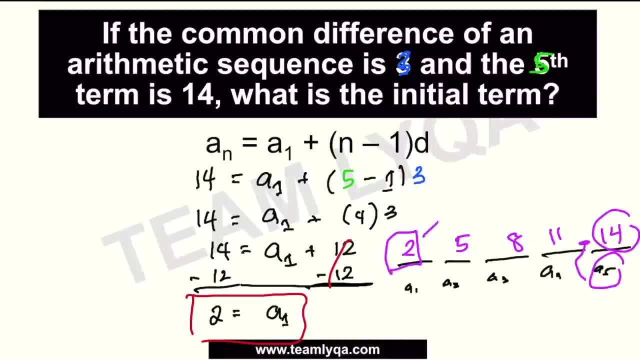 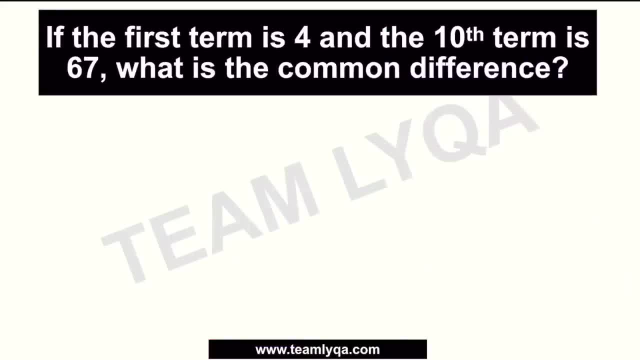 dyan, The 5th term is 14 if the initial term is 2, with a common difference of 3.. Okay, So again, the formula really comes in handy. Now, another possible question would be something like this, and I'm trying to cover: 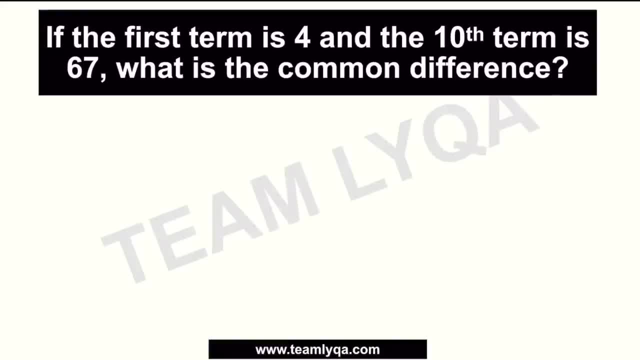 as much ground as possible para kung ano man yung ibibigay sa inyo, sa inyong module or sa inyong college entrance test? and again, yes, lumalabas yung ganitong klaseng tanong doon. 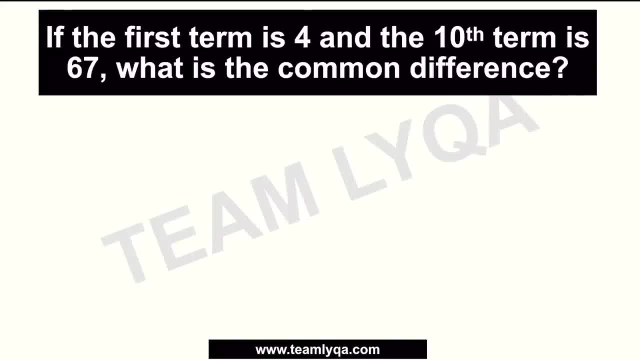 eh, ready kayo. If the 1st term naman daw is 4 and the 10th term is 67,. what is the common difference? Now again, you can fill in yung blanks, no Magsusulat ka ng 1,, 2,, 3,, 4,, 5,. 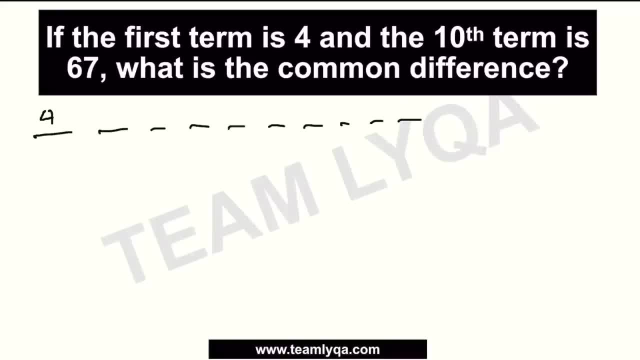 6,, 7,, 8,, 9,, 10.. Tas susulat mo dito yung 4, susulat mo to yung 67,. tas sumukan mo hulaan kung alin yung mga nandyan or 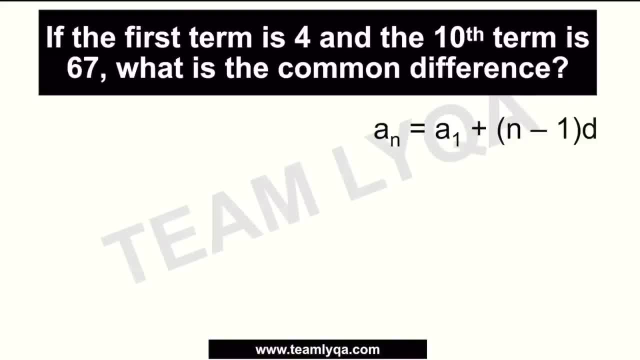 you can just use the formula: Okay, So ang ating a sub n, that would be the 10th term, which is 67. So lalagay natin dito: 67 is equal to the 1st term. 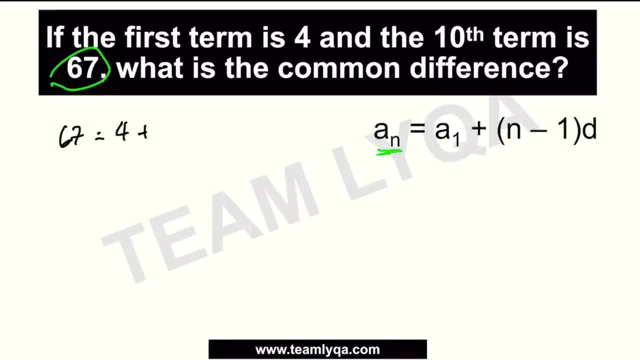 which is 4 plus yung number, so 10th term sya. so this will be 10 minus 1 times the d, na hindi natin alam ngayon. So solve lang natin ito: 67 is equal to: 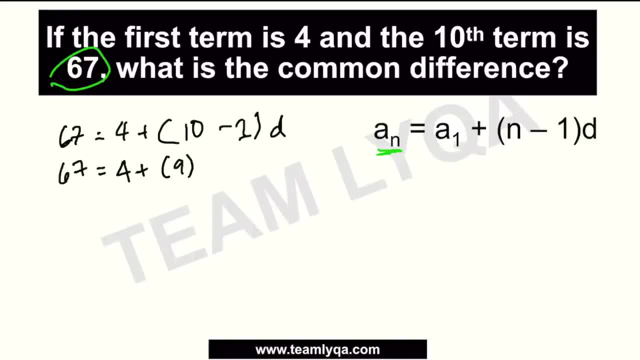 4 plus 9d 67. yulipat natin yung 4 dito sa kabilang side, So magiging 67 minus 4 is equal to 9d. 67 minus 4 is 63 is equal to 9d. 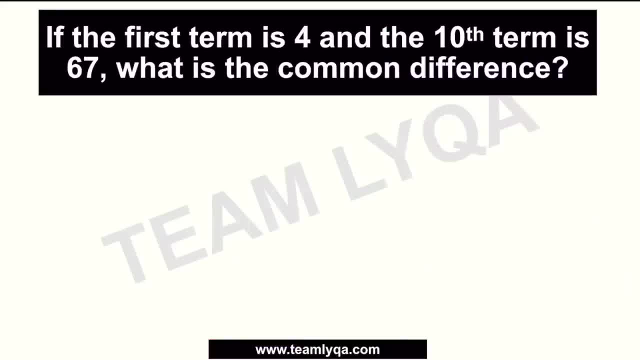 Okay, So again, the formula really comes in handy. Now, another possible question would be something like this, And I'm trying to cover as much ground as possible para kung ano man yung ibibigay sa inyong modules or sa inyong columns: 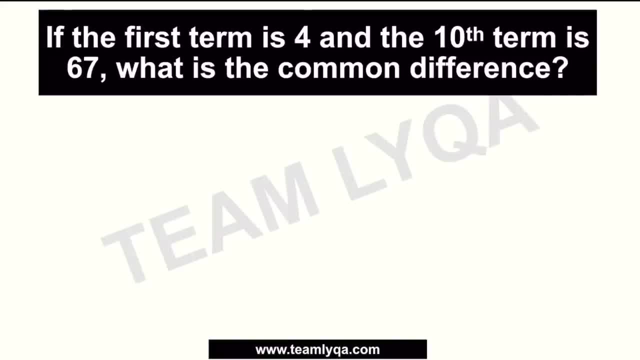 College entrance test. And again, yes, lumalabas yung ganitong klaseng tanong doon, Eh ready kayo. If the 1st term naman daw is 4 and the 10th term is 67,, what is the common difference? 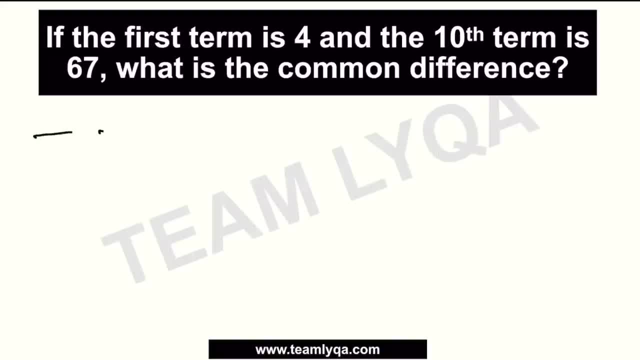 Now again you can fill in yung blanks. no Magsusulat ka ng 1,, 2,, 3,, 4,, 5,, 6,, 7,, 8,, 9,, 10.. 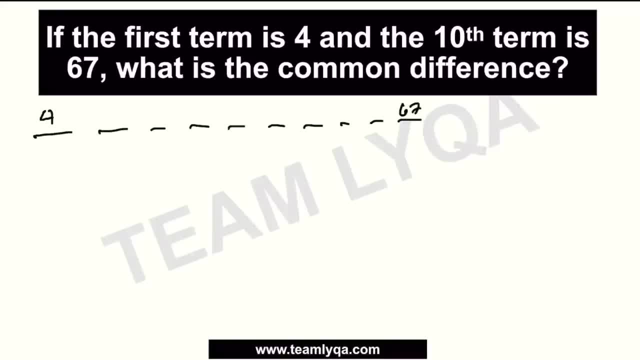 Tapos susulat mo dito yung 4.. Susulat mo dito yung 67.. Tapos sumukan mo hulaan kung alin yung mga nandyan, Or you can just use the formula. 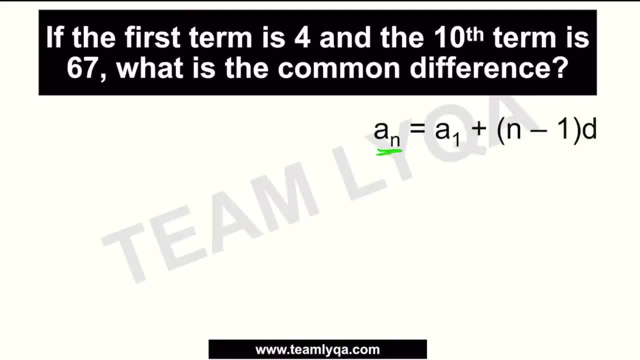 Okay, So ang ating a sub 8. And that would be the 10th term, which is 67.. So nalagay natin dito: 67 is equal to the 1st term, which is 4,, plus yung number. 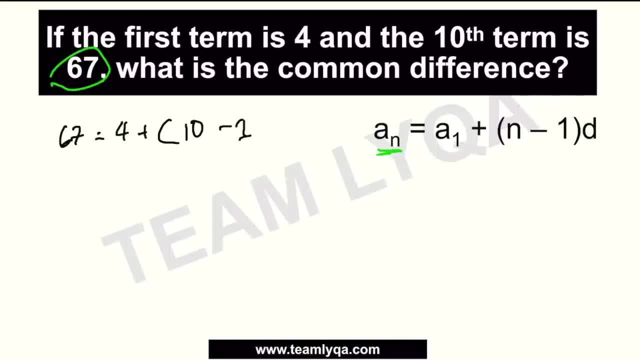 So 10th term siya. So this will be 10 minus 1 times the d na hindi natin alam ngayon. So solve lang natin. ito: 67 is equal to 4 plus 9d. 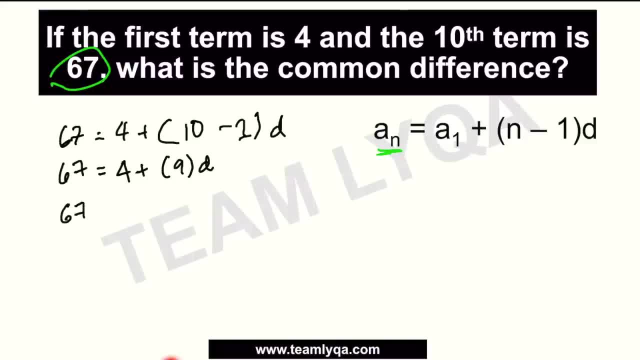 67, yulipat natin yung 4 dito sa kabilang side So magiging 67 minus 4 is equal to 9d. 67 minus 4 is 63, is equal to 9d. 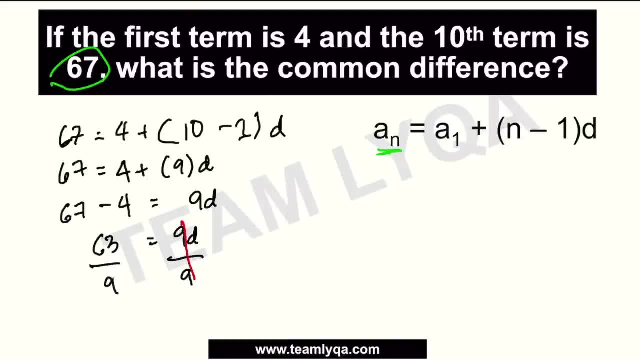 Divide natin both sides by 9.. Makakancel, ito 63 divided by 9 is 7.. So 7 is equal to d 7, ang common difference niya. Now again, if you want to check, just to make sure: 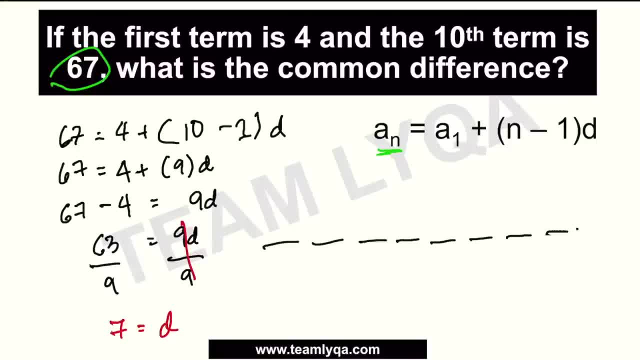 1,, 2,, 3,, 4.. 5,, 6,, 7,, 8,, 9,, 10.. 1st term is 4.. Kung ang common difference ay 7.. The next one will be 11.. 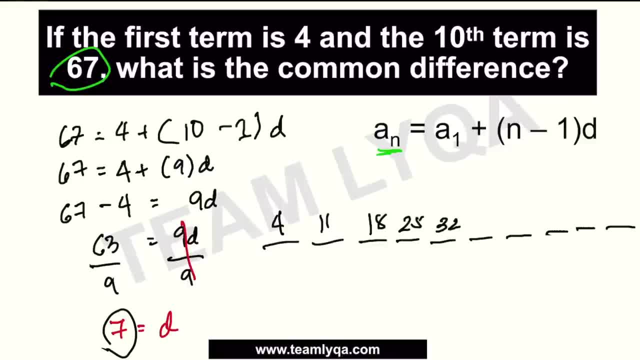 This will be 18.. 25,, 32,, 39,, 46.. 53,, 60, and 67.. So this is the 10th term, Tama tayo dyan So correct yung common difference na 7.. 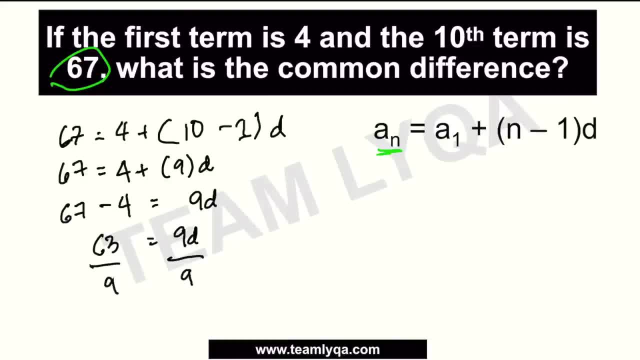 divide natin both sides by 9, makakancel ito 63 divided by 9 is 7. so 7 is equal to d 7. ang common difference nya now again, if you want to check just to make sure: 1,, 2,, 3. 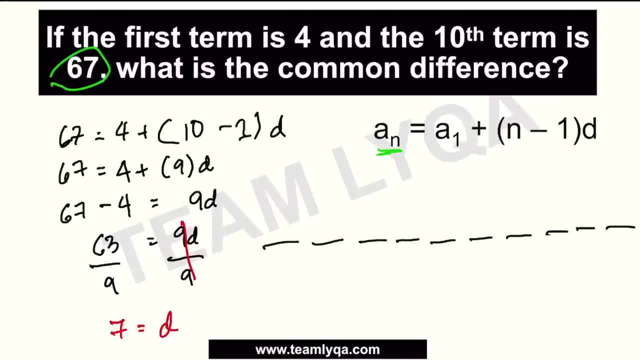 4,, 5,, 6, 7,, 8, 9, 10. 1st term is 4. kung ang common difference ay 7, the next one will be 11. this will be 18, 25,, 32. 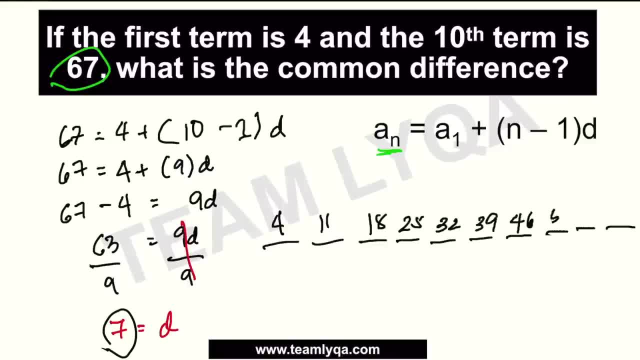 39,, 46, 53, 60 and 67, so this is the 10th term tama tayo dyan, so correct yung common difference na 7. so again very handy yung ating formula, lalo na kung malalaki yung mga numbers. 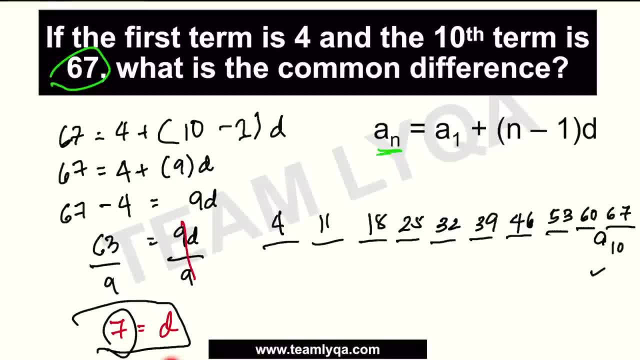 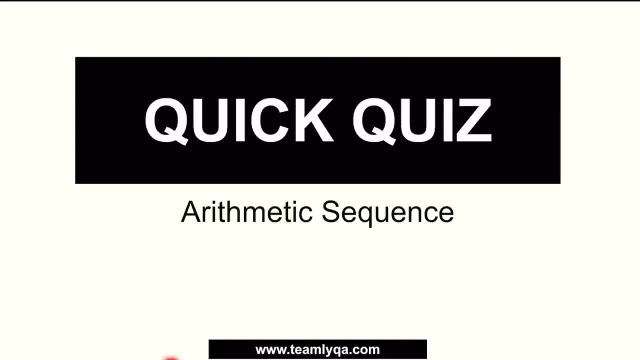 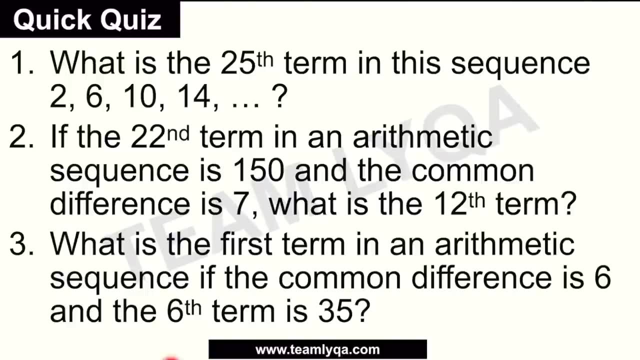 that we're dealing with. so I want you to try your handout by solving these 3 problems. if you're ready with your pen and paper, sa ating quick quiz. your timer starts now. alright, let's see how you did. let's start with the first problem. 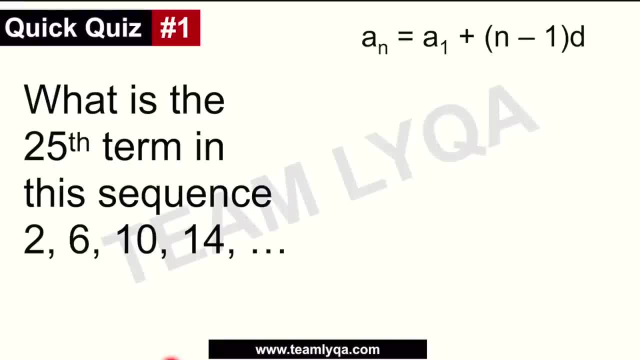 sabi: what is the 25th term in this sequence? now again, ang hinahanap is yung a sub 25 or the 25th term. that would be this, and then yung a sub 25 is equal to first term. natin is 2. 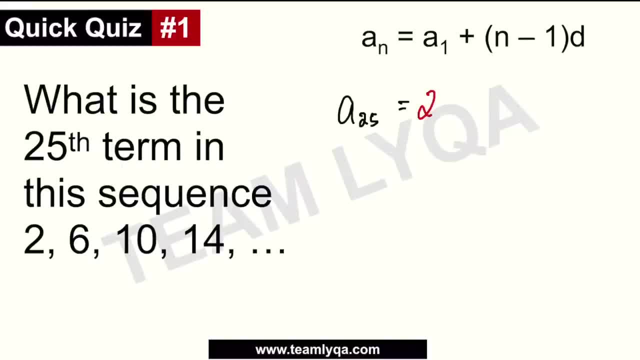 so susulat lang natin yung 2 plus yung ating n, which is 25, kasi 25th term ang hinahanap natin. so that would be 25 minus 1 times the common difference. and here we can find it by: 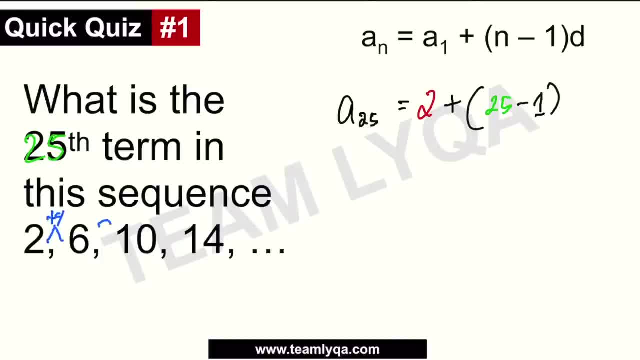 looking at the numbers, so 2 to 6, that is plus 4, this is plus 4 and another plus 4, so that would be 4. solve lang natin. 25th term is equal to 2 plus 24 times 4. 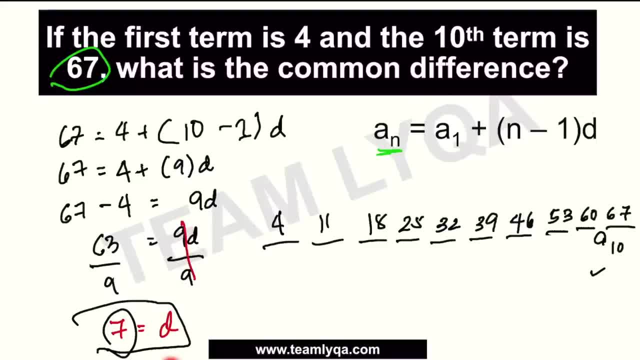 So again, very, Very handy yung ating formula: Lalo na kung malalaki yung mga numbers that we're dealing with. So I want you to try your hand out by solving these three problems, If you're ready, with your pen and paper. 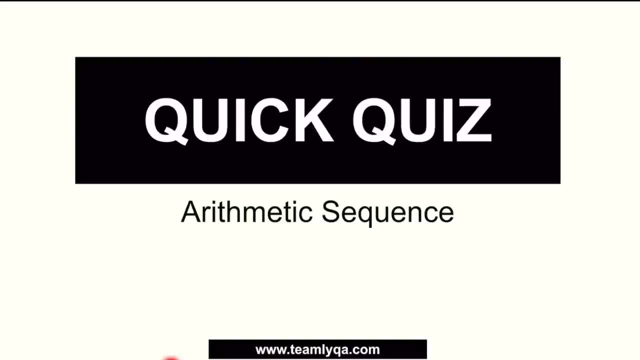 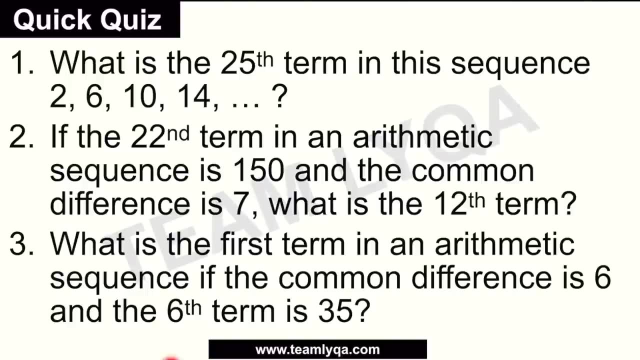 Sa ating quick quiz. your timer starts now. 🎵 🎵, 🎵, 🎵, 🎵, 🎵, 🎵, 🎵, 🎵, 🎵, 🎵, 🎵, 🎵, 🎵. 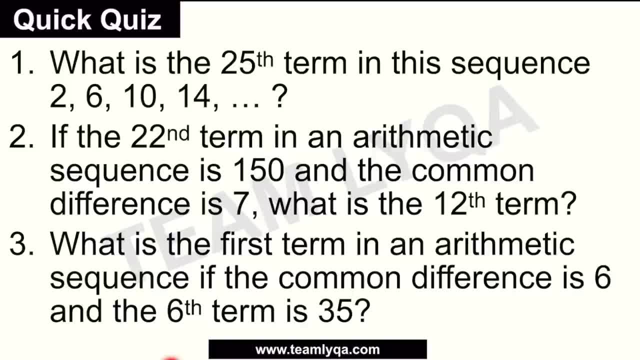 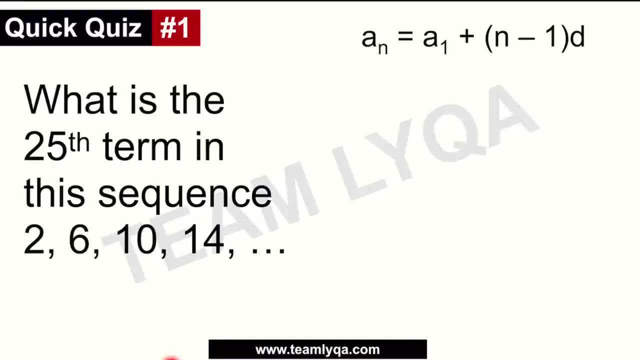 🎵 🎵. Alright, let's see how you did. Let's start with the first problem, Sabi: what is the 25th term in this sequence? Now, again, ang hinahanap is yung A sub 25 or the 25th term. 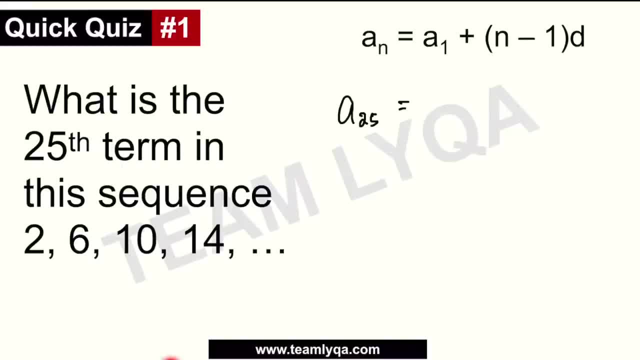 That would be this: It's equal to First term natin is 2.. So susulat lang natin yung 2 plus yung ating n, which is 25, kasi 25th term ang hinahanap natin. 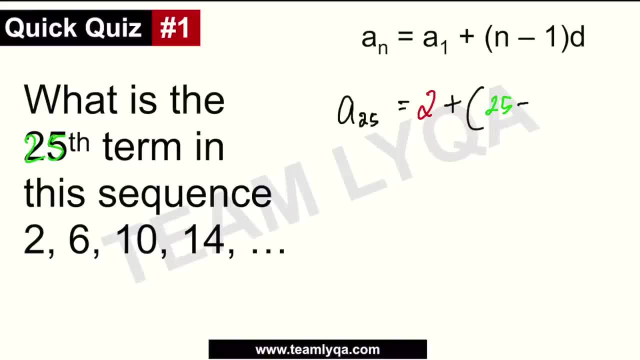 So that would be 25 minus 1 times the common difference. and here we can find it by looking at the numbers. So 2 to 6, that is plus 4.. This is plus 4 and another plus 4.. So that would be 4.. 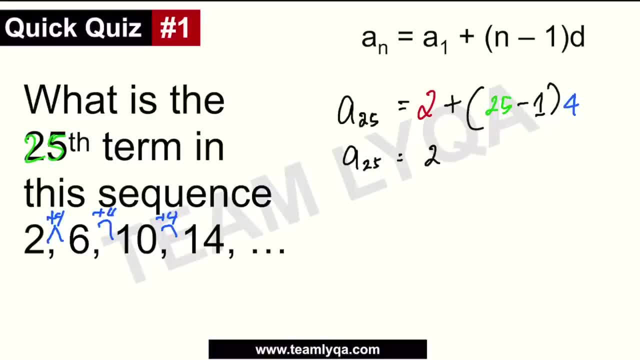 Solve lang natin. 25th term is equal to 2 plus 24 times 4.. So that would be 2 plus 24 plus 4, we can solve it like this: Ang apat na 20 ay 80.. 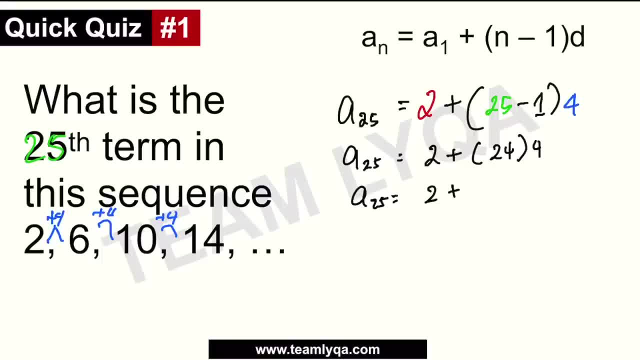 Ang apat na 4 ay 16.. So 80 plus 16 is 96.. So the 25th term is 98.. Okay, Yan ang ating sagot. Okay Now, next question, we have this: 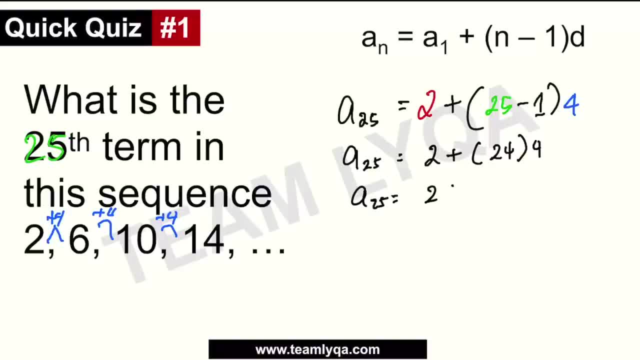 so that would be 2 plus 24 plus 4, we can solve it like this: ang apat na 20 ay 80, ang apat na 4 ay 16. so 80 plus 16 is 96. so the 25th term is: 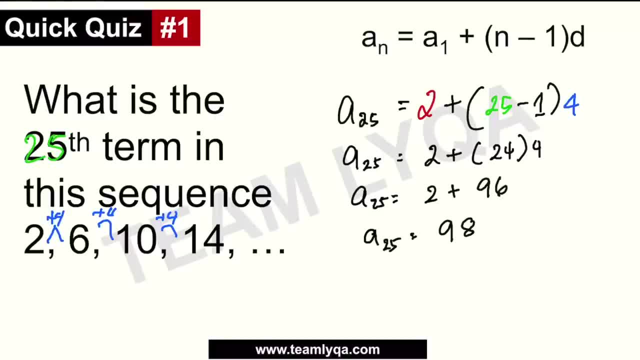 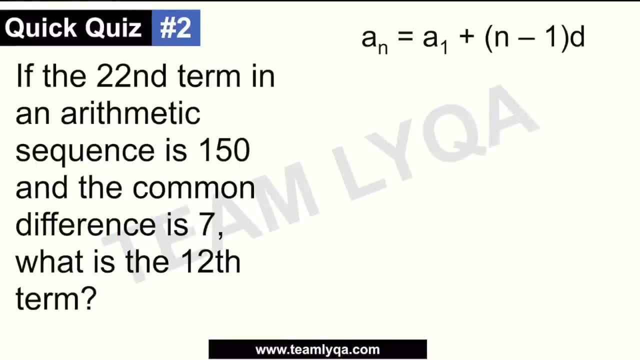 98. okay, yan ang ating sagot. okay now, next question, we have this: if the 22nd term in an arithmetic sequence is 150 and the common difference is 7, what is the 12th term? now, substitute lang natin again ang binibigay na sa atin. 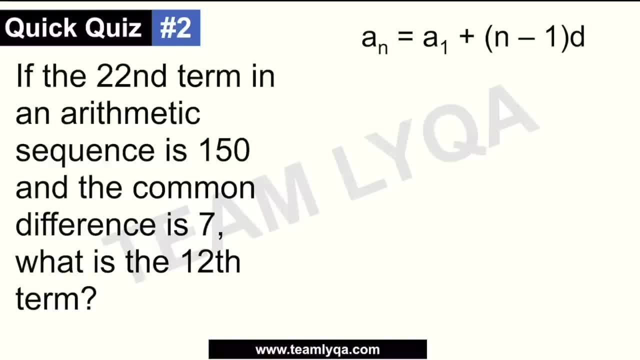 is yung 22nd term. so we can look at it this way: yung a sub 22 is 150. okay, so yun na agad ilalagay natin: 150 is equal to ang a sub 1, hindi natin alam. 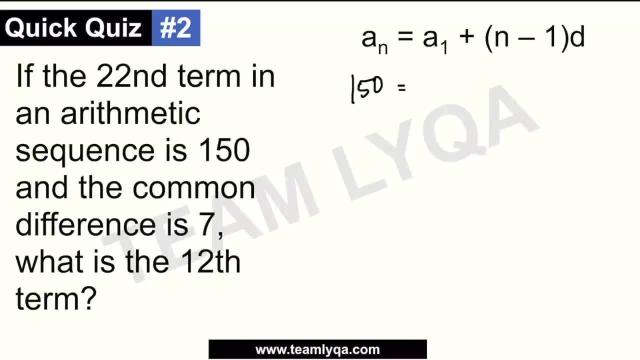 but we can leave it at that. so iwan muna natin sya as a sub, 1 plus, and then you have the n. in this case, again, we started with the 22nd term, so lagay natin 22 minus 1, tapos yung ating d. 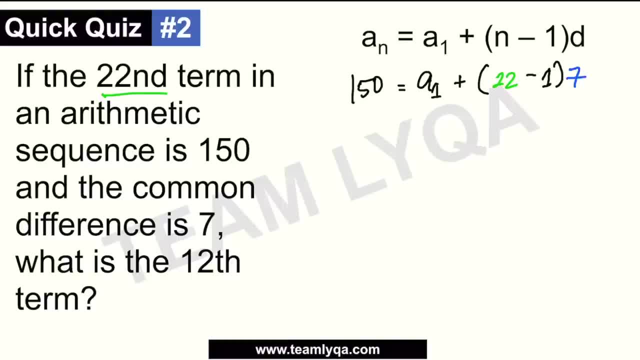 is the common difference, which is 7. okay, okay, this is the common difference, which is 7. okay, this time ito lang muna yung given natin isa-solve, muna natin yung first term para makuha natin yung. 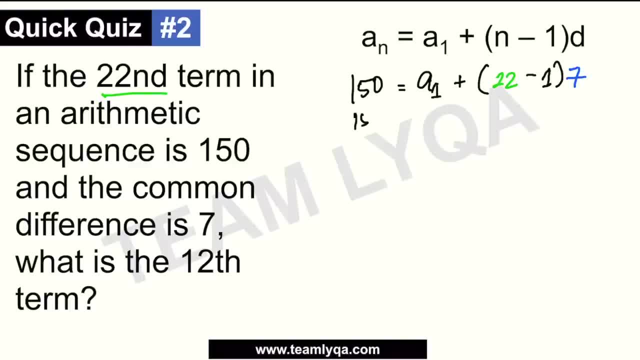 12th term. now 150 is equal to a sub 1 plus this is 21 times 7. so 150 is equal to plus 21 times 7, which is 20 times 7, 140 plus 1 times 7, 147. 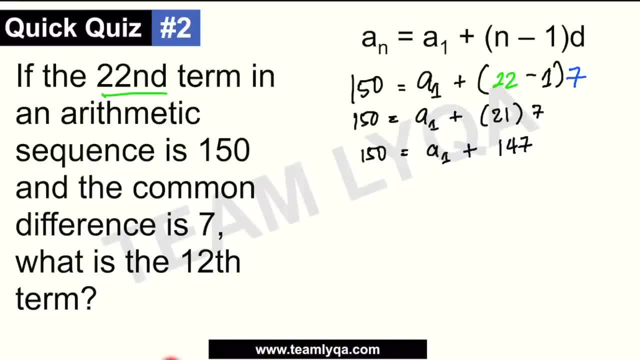 ako naguguluhan kayo dun sa explanation ko nayon, so I'm just using yung technique natin sa multiplying ng numbers. ililink ko rin dito yung video if you want to watch that now. using this we can get to a sub 1 or the initial term. 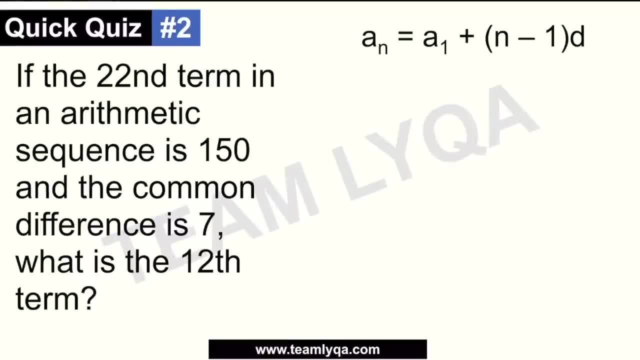 If the 22nd term in an arithmetic sequence is 150 and the common difference is 7,, what is the 12th term? Now substitute lang natin Again: ang binibigay na sa atin is yung 22nd term. 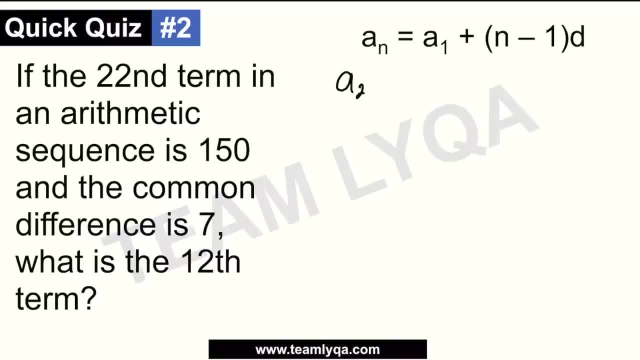 So we can look at it this way: Yung A sub 22 is 150.. Okay, So yan na agad ilalagay natin: 150 is equal to Ang A sub 1, hindi natin alam. 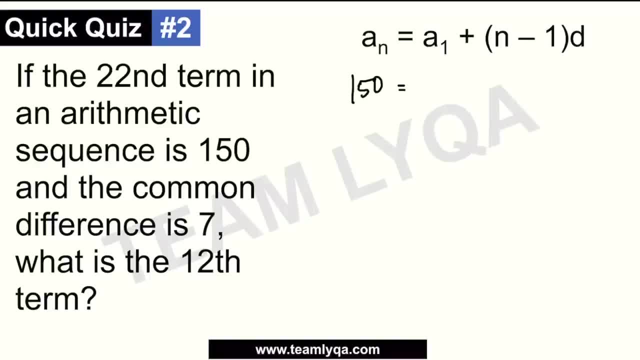 But we can leave it at that. So iwan muna natin siya as A sub 1. Plus. And then you have the N. In this case, again, we started with the 22nd term, So ilagay natin 22.. 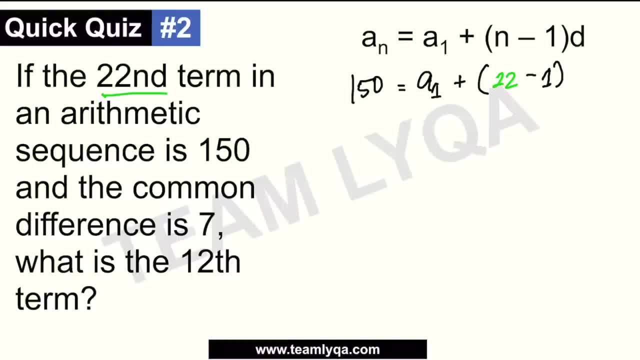 Minus 1.. Tapos, yung ating D is the common difference, which is 7.. Okay, This time ito lang muna yung given natin. Isosolve muna natin yung first term para makuha natin yung 12th term. 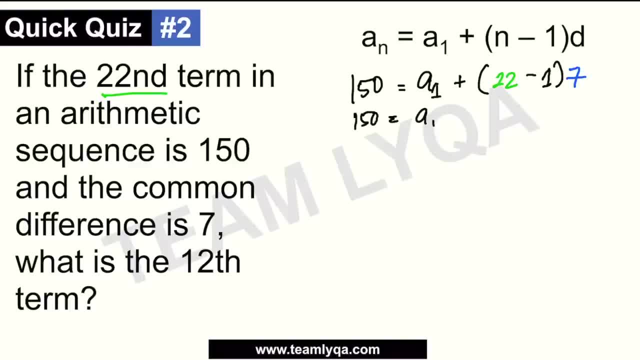 Now 150 is equal to A sub 1 plus this is 21 times 7.. So 150 is equal to plus 21 times 7, which is 20 times 7, 140 plus 1 times 7, 147.. 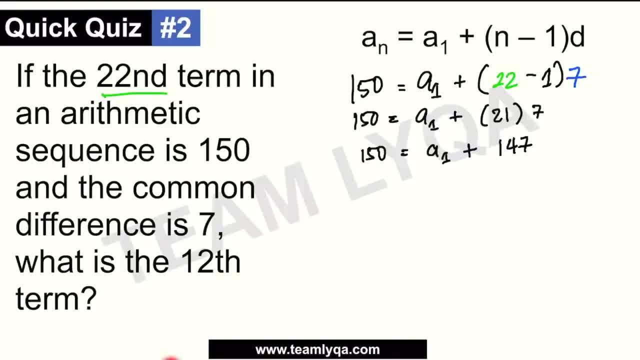 Now, kung naguguluhan kayo dun sa explanation. I'm just using yung technique natin sa multiplying ng numbers. Ililink ko rin dito yung video if you want to watch that Now. using this we can get to A sub 1 or the initial term. 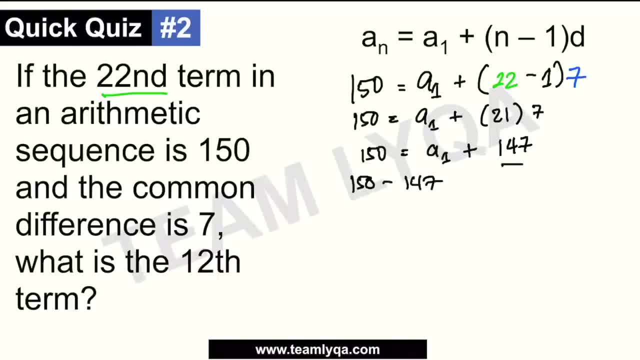 150, kasi minus 147, which is: this is equal to A sub 1. And this is 3.. So ibig sabihin nun, ang initial term natin ay 3.. Now, now that alam na natin yung initial term, we can now solve for the 12th term. 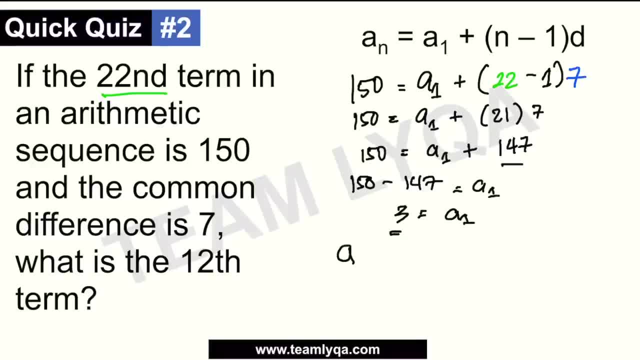 Now, how do we do that? We just use the formula again, So A- this time the 12th term- is equal to A sub 1, which is 3.. Nakasasolve natin kanina Plus yung N. this time we're looking for the 12th. 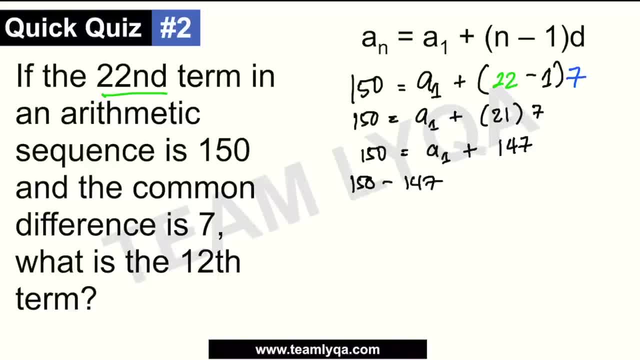 150, kasi minus 147, which is: this is equal to a sub 1 and this is 3, so ibig sabihin nun, ang initial term natin ay 3. now that alam na natin yung initial term, we can now solve for the 12th term. 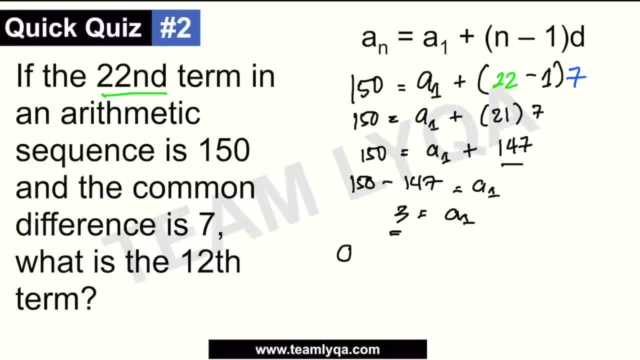 now, how do we do that? we just use the formula, so a- this time the 12th term- is equal to a sub 1, which is 3 plus yung n. this time we're looking for the 12th, so this will be 12. 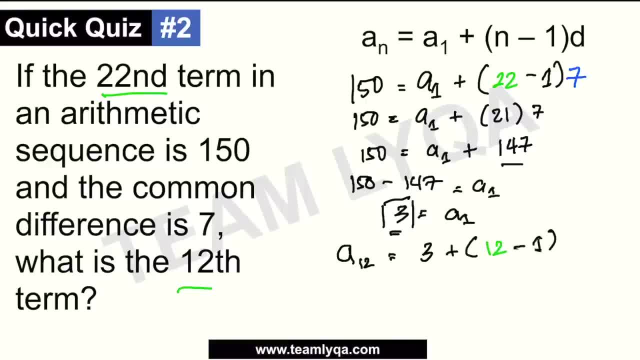 minus 1 times the difference, which is still 7. so that would be 3 plus 11 times 7, or 3 plus 77. so ibig sabihin nun, ang 12th term is 80. okay, sagot natin is 80. 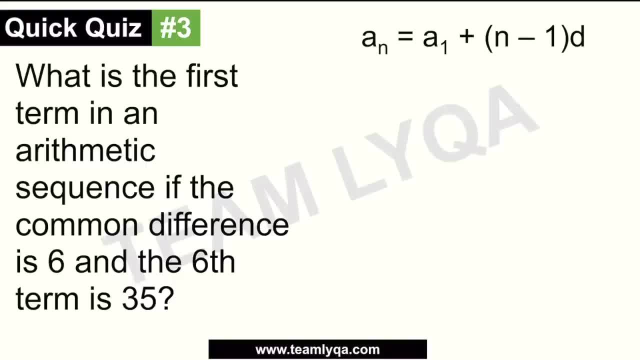 okay, now number 3: what is the first term in an arithmetic sequence if the common difference is 6 and the 6th term is 35? so again, kung yung a sub 6 ay 35, we can put it there, ang ating first term ay nawawala. 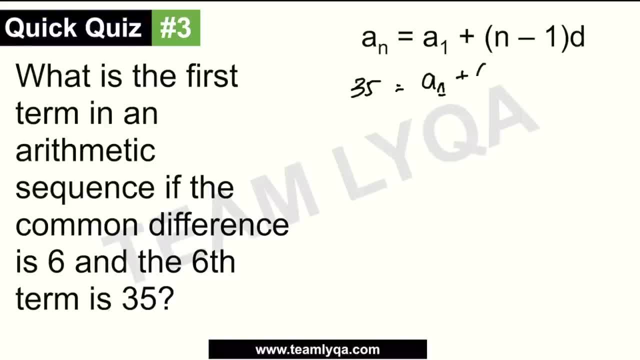 so we'll leave it at a sub 1 plus, and then yung n natin is 6 minus 1 times the common difference, which is also 6. okay, ito, yun binigay naman sya. okay, so we're going to solve for. 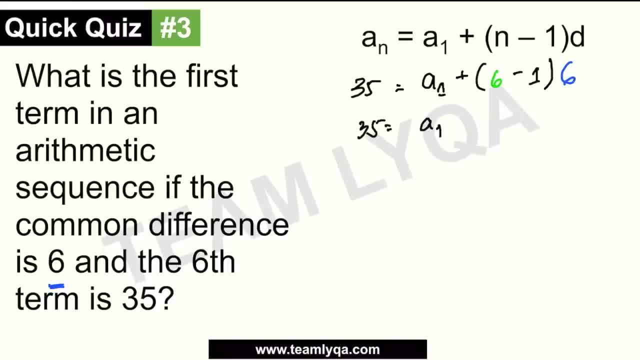 that 35 is equal to a sub 1 plus 5 times 6, so 35 is equal to a sub 1 plus 30. so para maiwan yung ating nawawala, yung nawawala, gagawin natin minus 30. 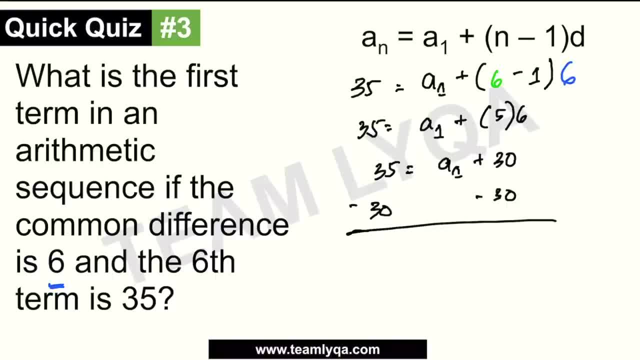 on both sides na lang, so we can do it like that. so this will be: 5 is equal to a sub 1 or the initial term, maka cancel kasi ito. kasi positive 30 plus negative 30 is 0, so ang first term natin. 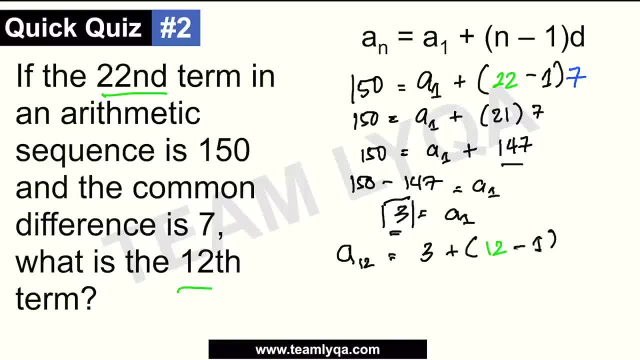 So this will be 12 minus 1 times the difference, which is still 7.. Okay, So that would be 3 plus 11 times 7, or 3 plus 7.. So ibig sabihin nun, ang 12th term is 80.. 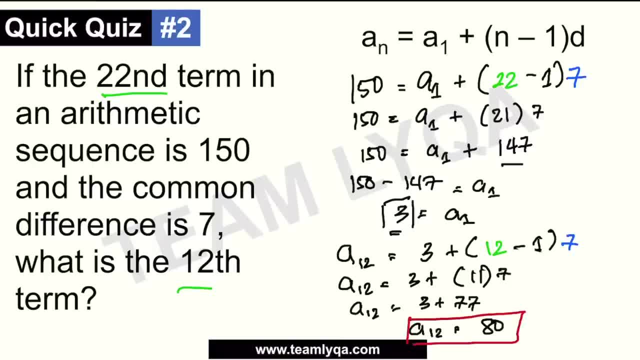 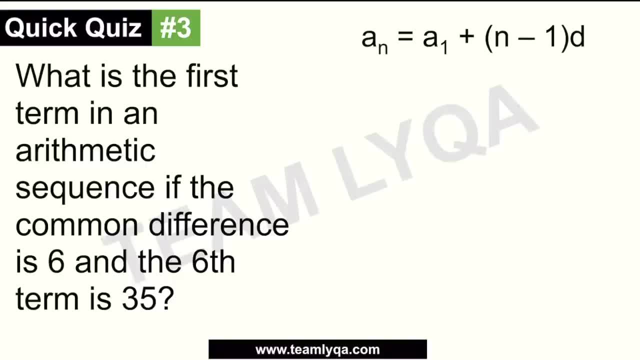 Okay, Sagot natin is 80.. Okay, now number 3.. What is the first term in an arithmetic sequence if the common difference is 6 and the 6th term is 35?? So again, kung yung A sub 6 ay 35, we can put it there. 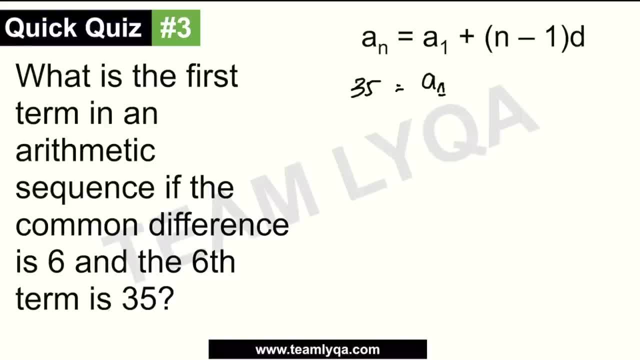 Ang ating first term ay nawawala, So we'll leave it at A sub 1. Plus. And then yung N natin is 6 minus 1 times the common difference, which is also 6.. Okay, Ito yun. 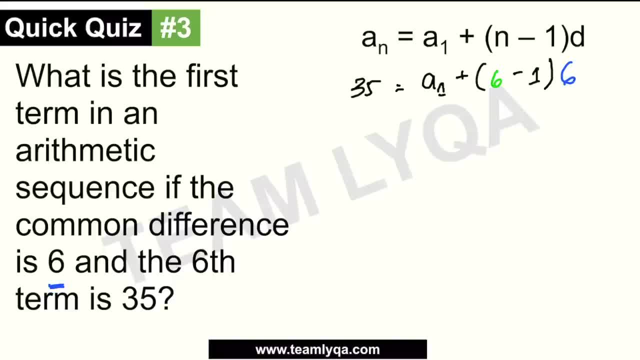 Binigay naman, siya, Okay, So we're going to solve for that. 35 is equal to A sub 1 plus 5 times 6.. So 35 is equal to A sub 1 plus 30.. 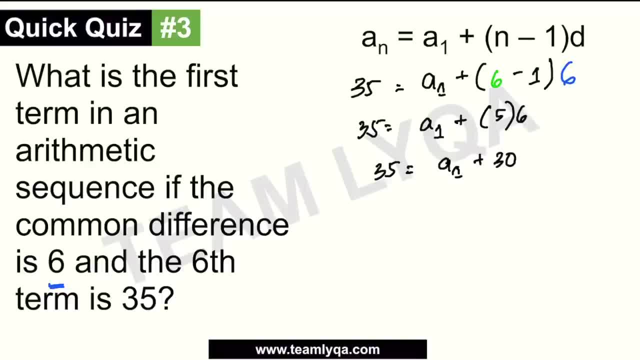 So para maiwan yung Ating nawawala, Gagawin natin minus 30 on both sides na lang, So we can do it like that. So this will be: 5 is equal to A sub 1 or the initial term. 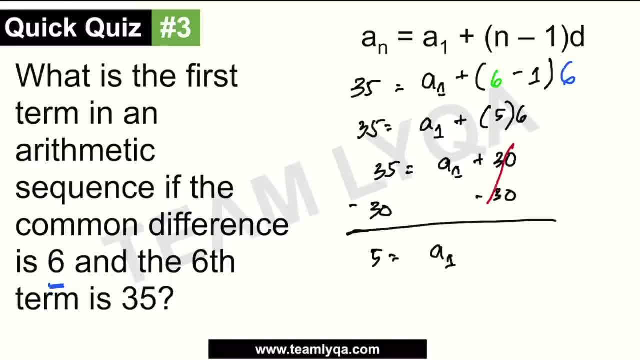 Maka-cancel kasi ito. kasi positive 30 plus negative 30 is 0.. So ang first term natin is 5.. Okay Now I hope you got all of the three questions correctly. If you didn't, that's okay. 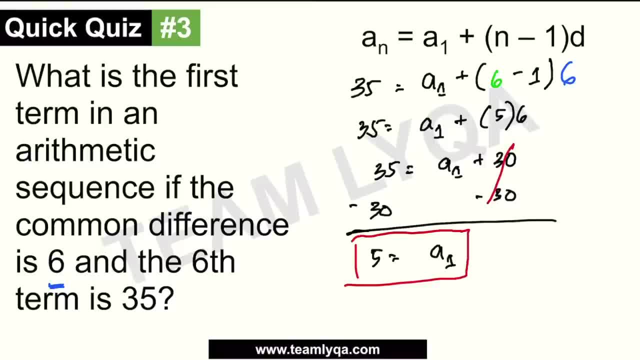 Medyo challenging yung number 2 natin. But I'm going to be posting more questions naman My Instagram account, So if you don't follow me yet, you can follow me at Laika Maravilla on Instagram for more quick quizzes. 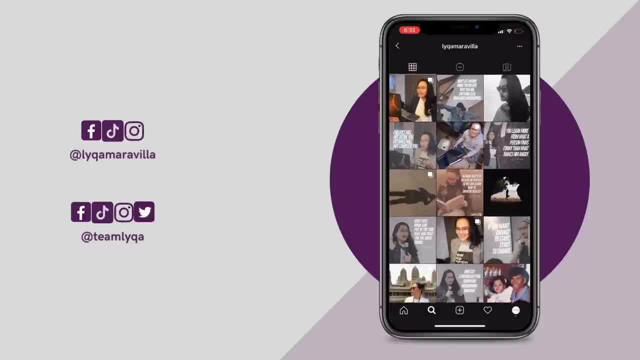 You will find out right away kung tama kayo. Kasi, pag tinap ninyo yung sagot dun sa ating Instagram story, manalaman ninyo if you're going to have confetti or ibibigay din sa inyo kung ano yung tamang sagot. 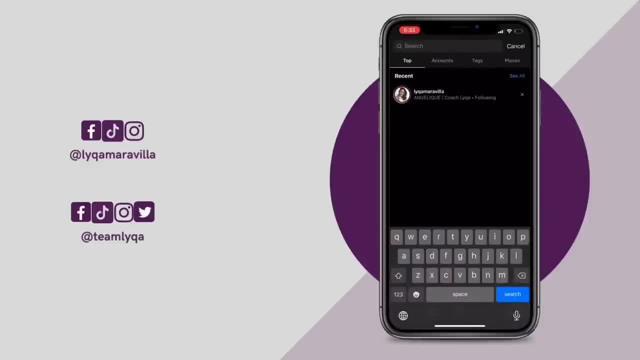 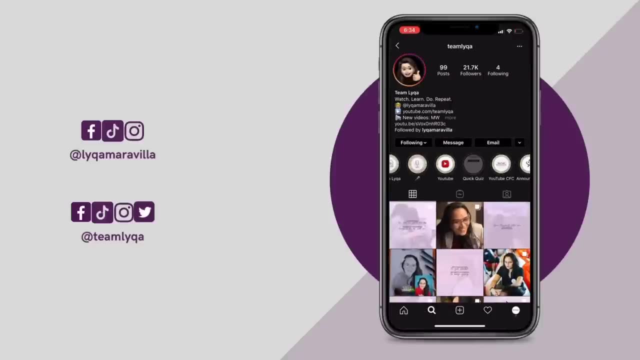 Okay, You can also follow me at Team Laika for the throwback quick quiz questions. We already covered a lot of topics sa 900 plus videos natin sa channel na ito, So kung gusto nyo ng bagong refresher. 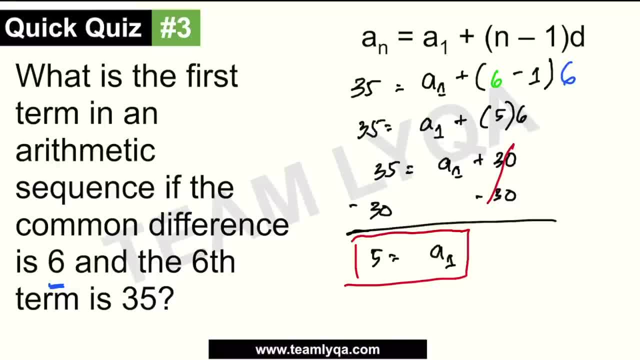 is 5. okay now. I hope you got all of the 3 questions correctly. if you didn't, that's okay, medyo challenging yung number 2 natin. but I'm going to be posting more questions naman on my Instagram account, so if you don't follow me yet, 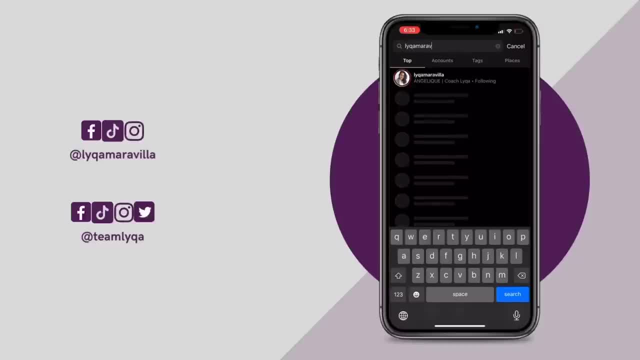 you can follow me at Laika Maravilla on Instagram for more quick quizzes. you will find out right away kung tama kayo. kasi, pag tinap ninyo yung sagot dun sa ating Instagram story, manalaman ninyo. 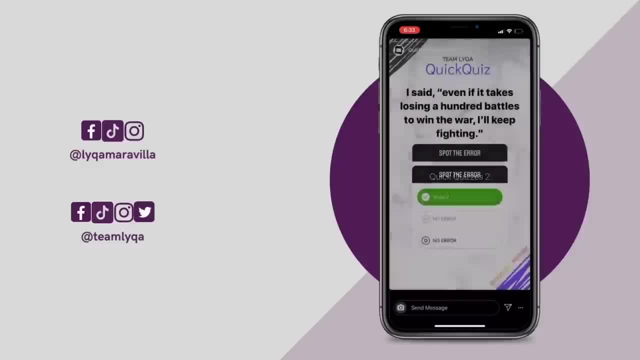 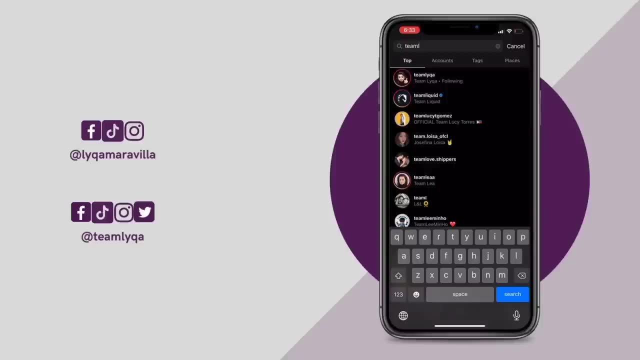 if you're going to have confetti or ibibigay din sa inyo. kung ano, yung tamang sagot. okay, you can also follow me at Team Laika for the throwback quick quiz questions. we already covered a lot of topics sa 900 plus videos. 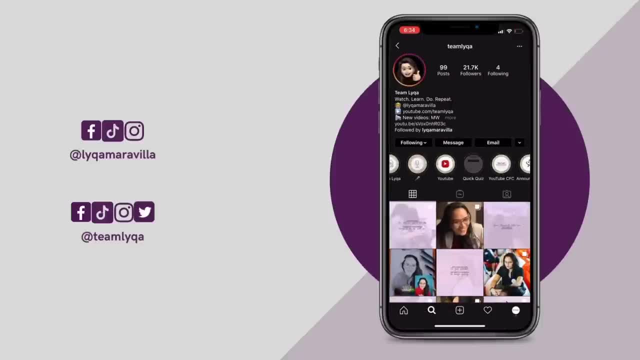 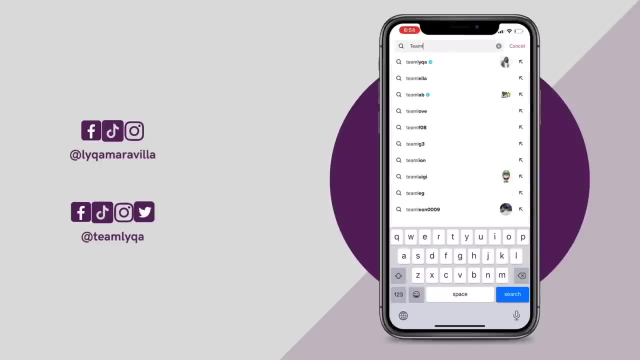 natin sa channel na ito. so kung gusto nyo ng bagong refresher, dun kayo mapupunta sa Team Laika on Instagram. you can also follow me on TikTok at Team Laika for the mga lessons nyo rin, yan, mga math language. 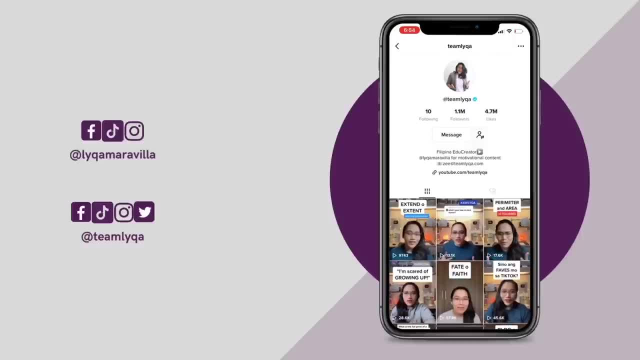 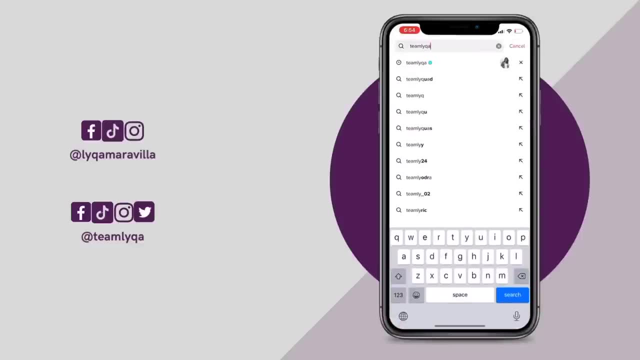 logic lessons, quick quizzes, na iba pa doon sa pinupost ka sa Instagram mga tutorials at marami pang iba. and if you want to get to know me a little bit better, yung aking personal channel or personal account sa TikTok. 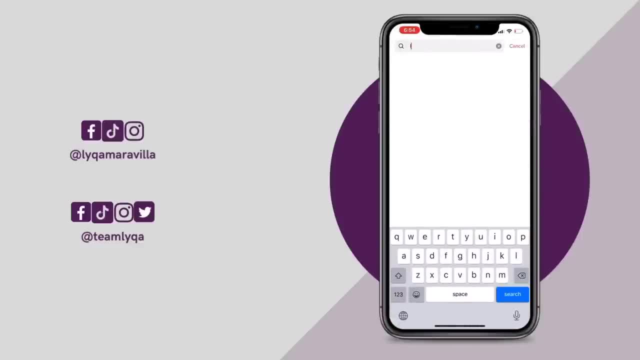 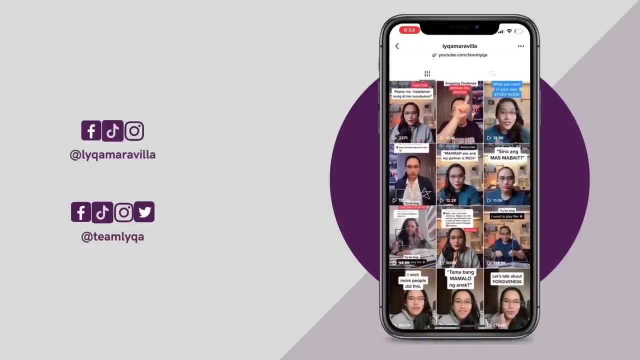 is at Laika Maravilla naman, where I post my motivational videos, tips, advice, mga ibang mga skits, at iba pang mga things that I just want to post. alright, I'll see you online. alright, I hope you understood me today if you did click thumbs up. 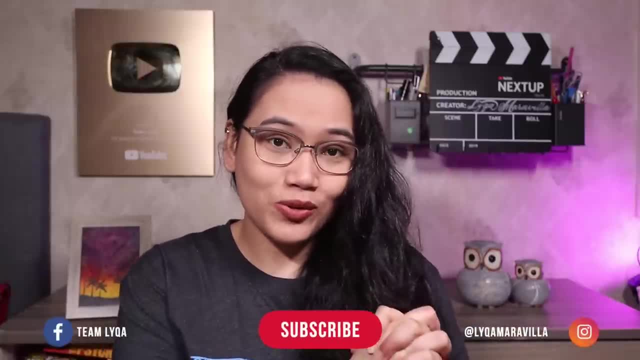 make sure that you share this video with your friends. saan lang ako mag-examine din sila. that way, mas marami tayong matutulungan and, as always, if you want to reach out to me directly, get reviewers that I made. join the online or live. 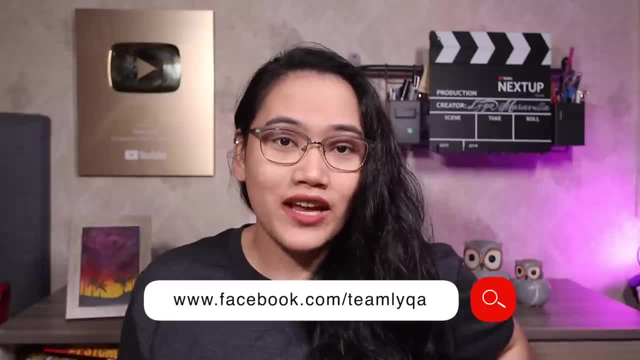 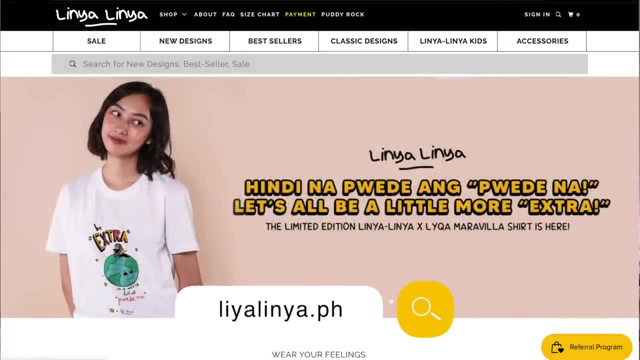 review events. you can go to wwwfacebookcom slash Team Laika if you want to get this shirt by Linya Linya PH or a super special collab shirt na Linya Linya X, Laika Maravilla. be extra in a world full of. 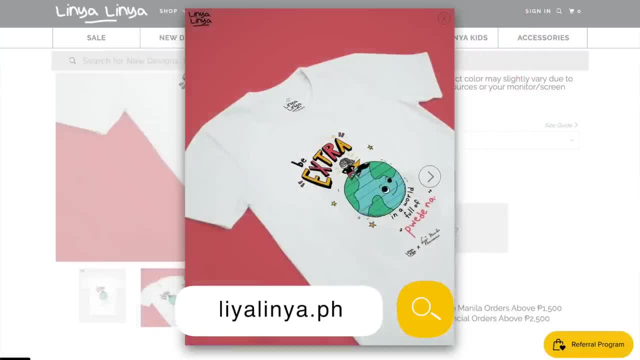 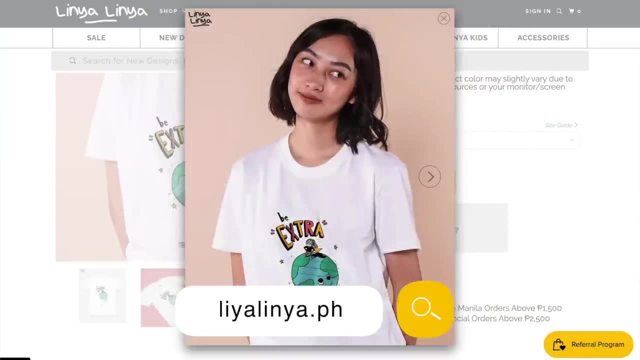 pwede na? you can go and check that out. pa rin sa Linya Linya dot PH and stay tuned until the end of the video to find yung ating super special din na discount code to get 10% off sa shirt na yan and other regular. 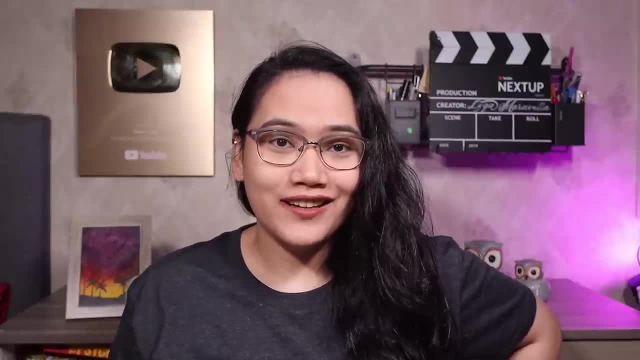 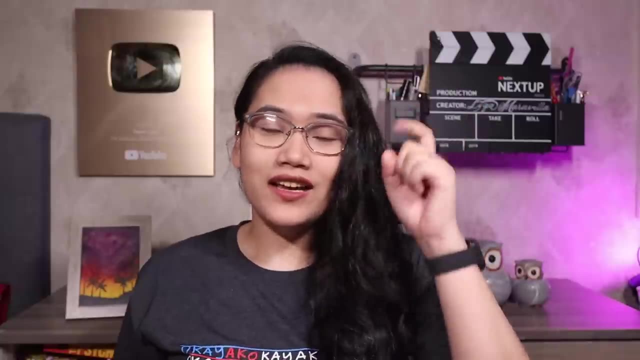 priced shirts sa Linya Linya dot. PH. alright subscribe. if you haven't yet hit that bell icon, we have more videos coming up and, as we always say sa channel na to never stop learning, adja adja kaya niyan. I'll see you in my next video. 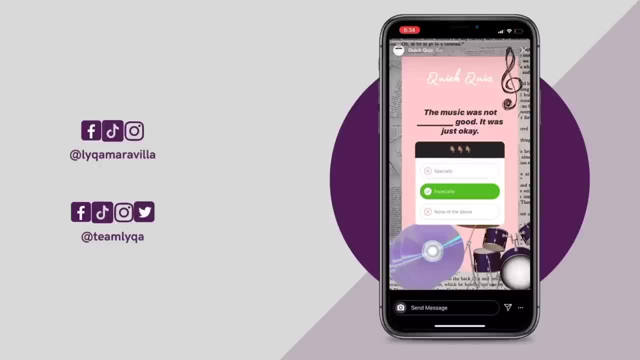 dun kayo mapupunta sa Team Laika on Instagram. You can also follow me at Team Laika on Instagram. You can also follow me at Team Laika on Instagram. You can also follow me on TikTok at Team Laika for the mga lessons niya rin yan. 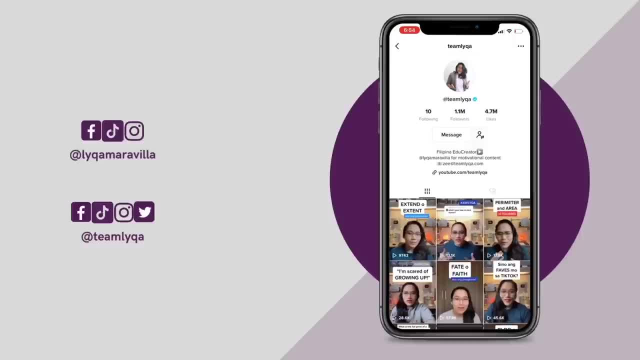 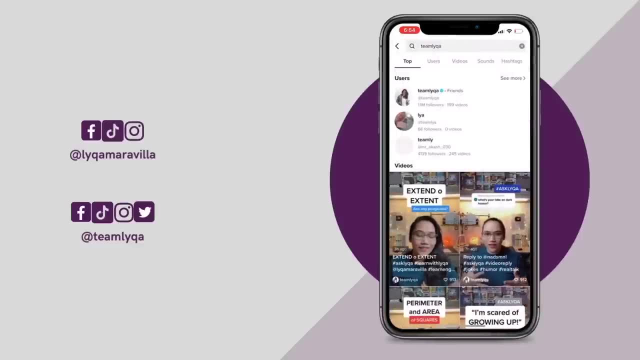 Mga math language logic lessons, quick quizzes, na iba pa doon sa pinupost ka sa Instagram Mga tutorials at marami pang iba. And if you want to get to know me a little bit better, yung aking personal channel or personal account sa TikTok. 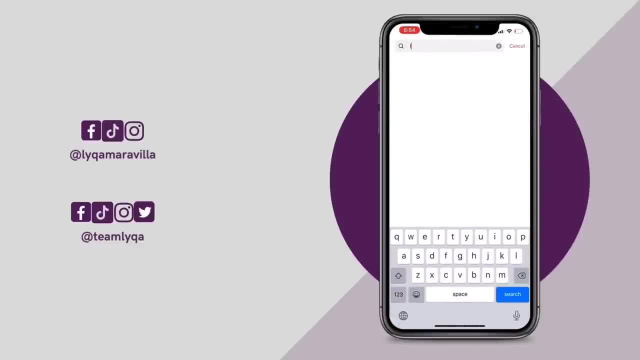 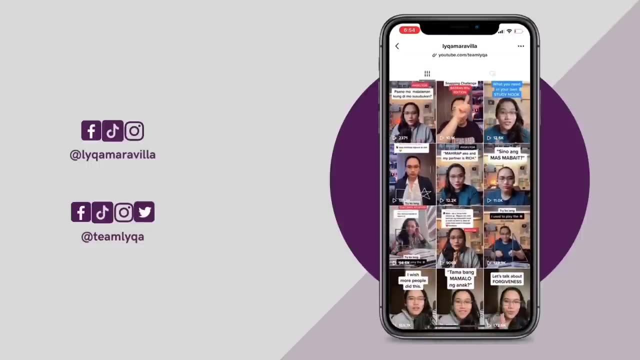 is at Laika Maravilla naman, where I post my motivational videos, tips, advice, mga ibang mga skits at iba pang mga things that I just want to post. Alright, I'll see you online. Alright, I hope you learned something today. 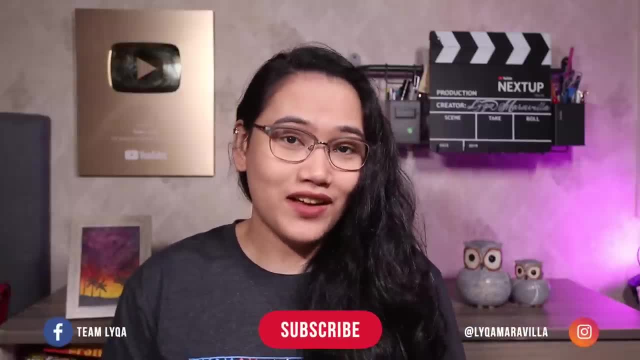 If you did click the subscribe button, Click thumbs up. Make sure that you share this video with your friends, sa ano lang mag-examine din sila. That way mas marami tayong matutulungan. And, as always, if you want to reach out to me directly. 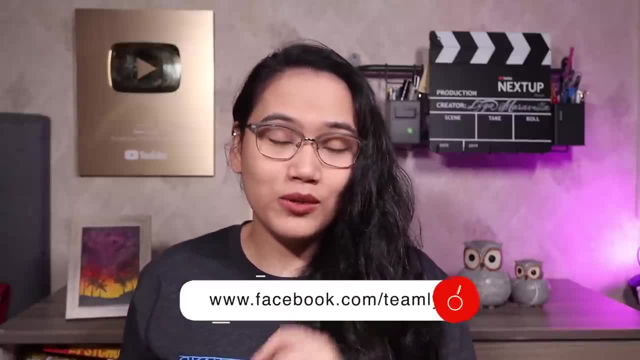 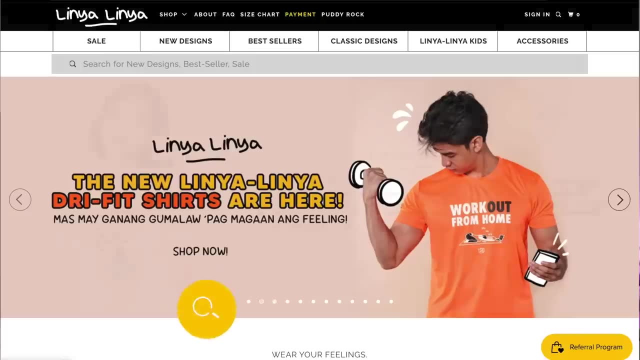 get reviewers that I may join the online or live review events. you can go to wwwfacebookcom slash Team Laika If you want to get this shirt by Linya Linya PH or a super special collab shirt na Linya Linya X, Laika Maravilla. 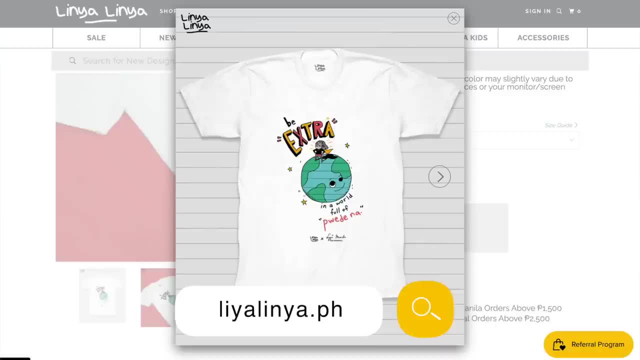 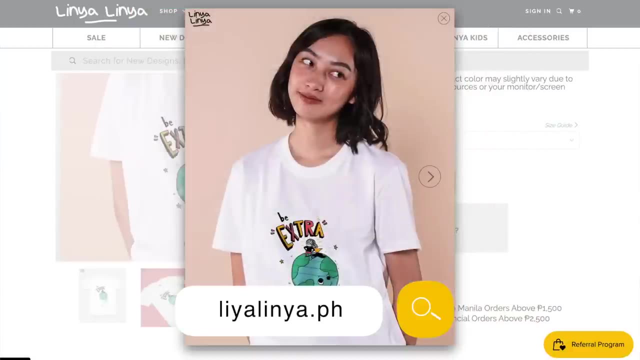 be extra enrolled full of Pwede Na. you can go and check that out pa rin sa LinyaLinyaph and stay tuned until the end of the video to find yung ating super special din na discount code to get 10% off sa shirt na yan. 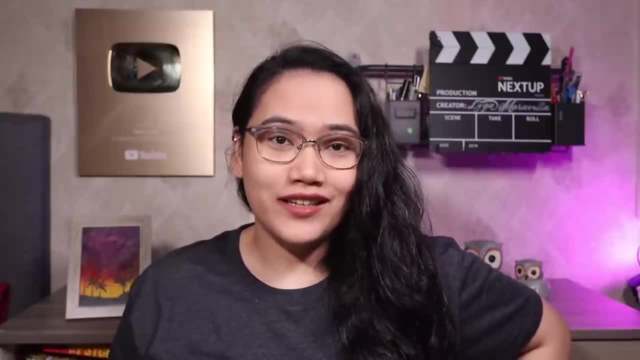 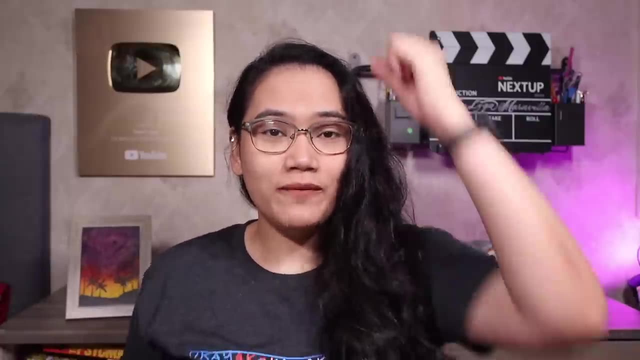 and other regular priced shirts. sa LinyaLinyaph Alright Subscribe. if you haven't yet Hit that bell icon, We have more videos coming up And, as we always say, sa channel na to never stop learning, Adja adja. 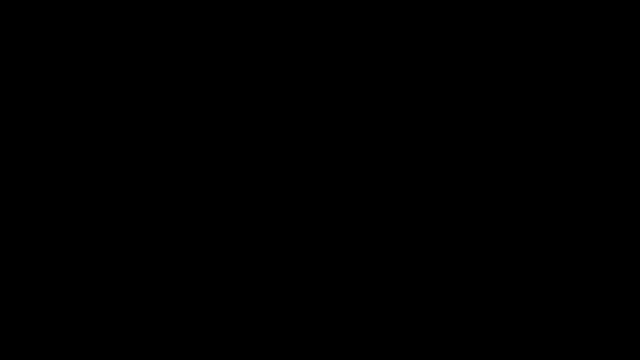 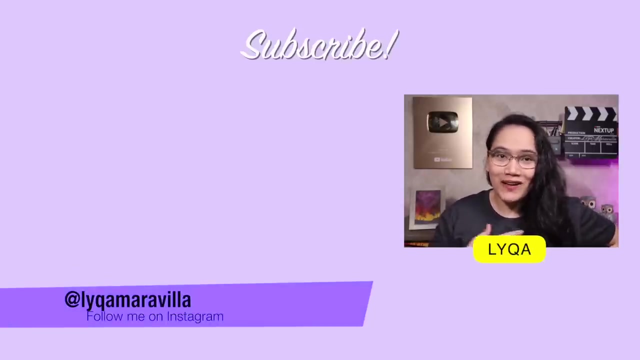 Kaya niyan. I'll see you in the next video And bye for now. Alright, now it's time for that super special discount code. It's really quite simple. It's LYQA Yung spelling ng aking pangalan. 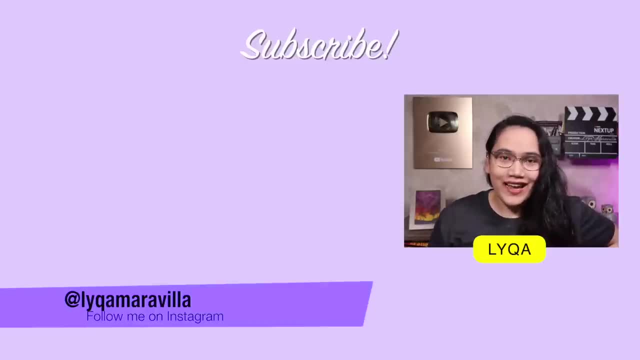 Again, it's LYQA Ha, hindi C or K, K or CK, And you will get 10% discount sa LinyaLinyaph. So mga bumili na ng shirts natin. Maraming salamat sa inyo. And salamat sa support ninyo lahat. I'll see you next time.